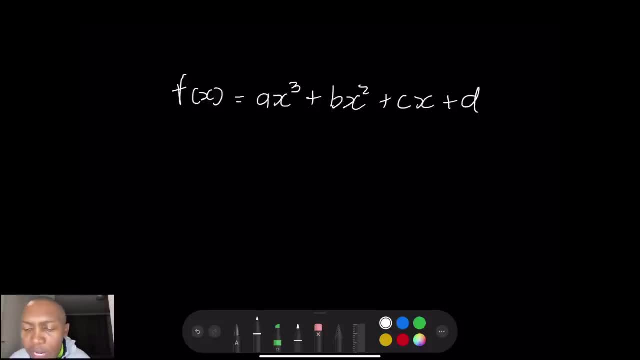 squared plus c, x plus d. all right, now let's first establish just a few things about our cubic functions, date methods and a half and minus x. okay, we are going to look what the following is. all right, we'd like to use this special formula that we use at this point: a and plus or minus greater than so. we would enjoy looking at this. anyway, i will give you the equations under second held when you visit a class. so the first things that we always notice is that, well, when the value of a meaning, the coefficient of x cubed, is greater than zero, now it will affect the shape of our graph. so how would our graph look like? so our graph would usually start with a local maximum and therefore follow a local and therefore follow a local. 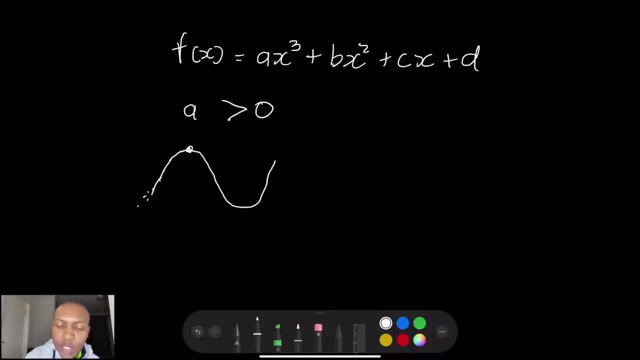 so what you'd see is that a graph would start with a one and then, years after years, we are one would actually start as an increasing function. okay, get to that maximum point there, all right, and then obviously have a minimum, okay, and of course, when the value of a is less than zero. 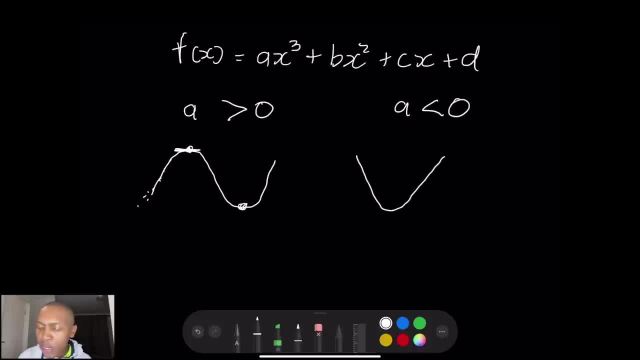 our graph would be shaped more or less in this way. okay, so you'd start, in this case, with the decreasing function, that starts with the local minimum and thereafter a maximum. okay, right now, here's a couple of things that i want us to actually, uh, just know about a cubic function. 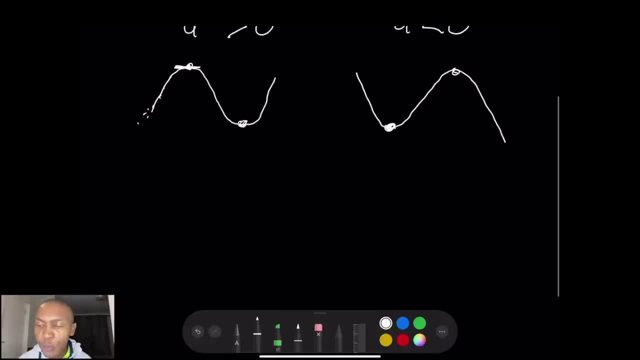 and please, i want you to remember this. uh, you know, for for calculus right now, how do you first of all determine- now we're going to talk about a couple of things here- how do you determine, or how do you find the local minimum and then after a maximum? okay, right now, here's a couple of things. 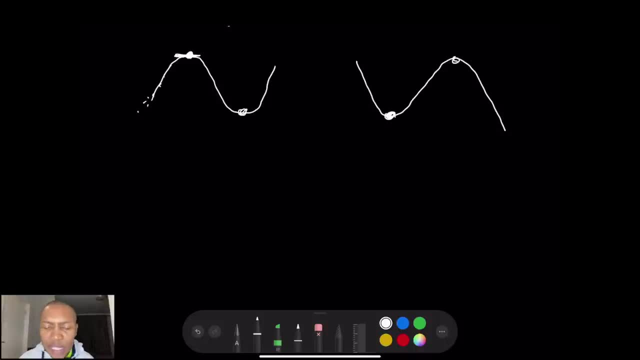 in fact, let's start with the very basic things. of course we know, just like we did for any other function, to find the y intercept. okay. so we always say x is equal to zero, okay. so obviously it means everywhere you see x, you are going to substitute a zero, all right, and that gives you your y. 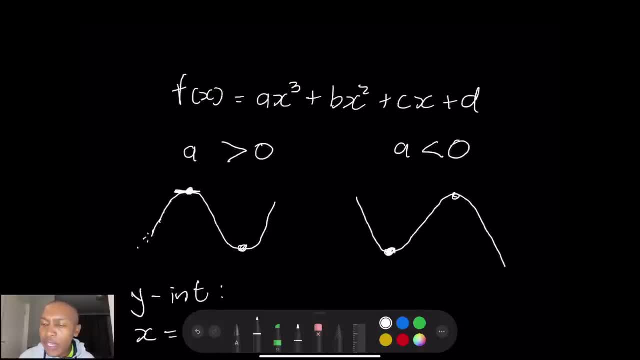 intercept. so if you've got your graph, in this case you know, or rather the equation of your graph in this manner, then it means the constant term, this d term actually gives you your, your y intercept. okay, right, and then obviously we do know how to get the. 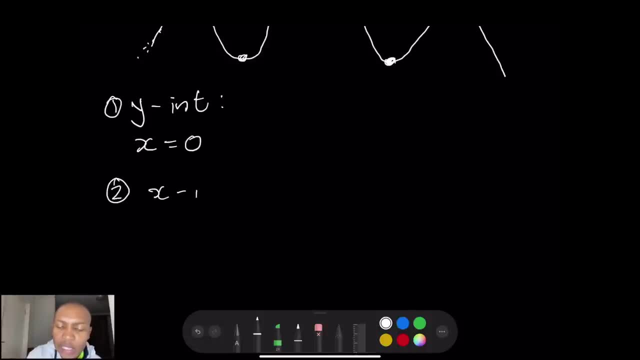 x intercept as well. so the second thing is the x intercept. of course we do know, at the x intercept, you know that x, or rather y rather, is equal to zero. so we know that y is equal to zero, zero. so you're going to take your equation, equate it to zero and of course you are going to 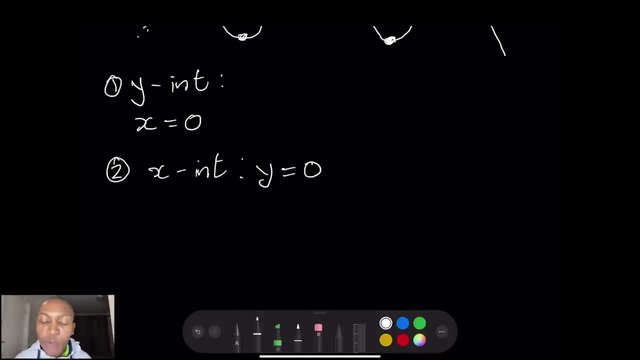 you know, factorize- okay, and of course that's why, in our previous lesson, we talked to you about synthetic division, in this case, so that you are able to get those factors right. okay, and number three. so now we want to know how to get the turning point. so how do we get the turning point? 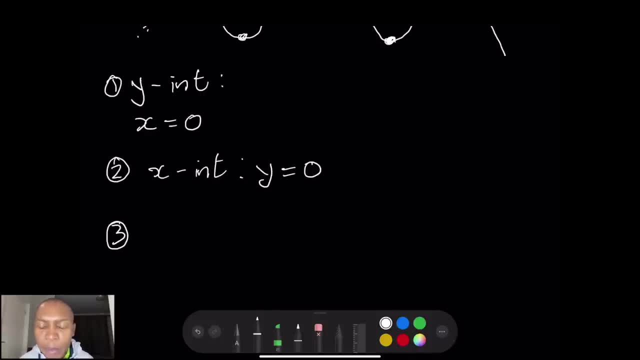 so how do we get our local minimum and how do we get the turning point? so how do we get the turning point, so how do we get our local minimum and maximum? and, of course, we're going to add some vocabulary to it. okay, you hear me talking about local minimum and maximum. in this case, all we simply do, 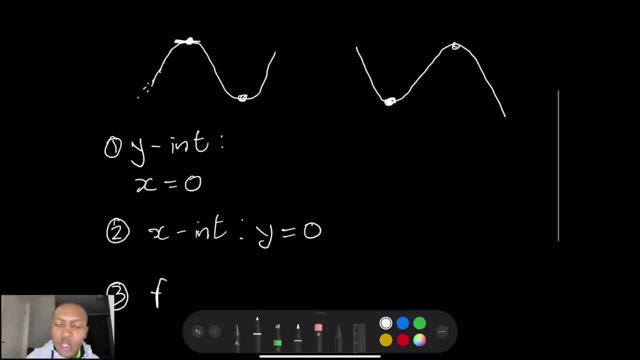 remember that when we what happens at your, you know your maximum point or your minimum point. well, this is where the gradient is essentially equal to zero. now let me just show you quickly about this, the shape of this graph. if i look at this graph over here, you can see that the gradient here is actually positive, right? 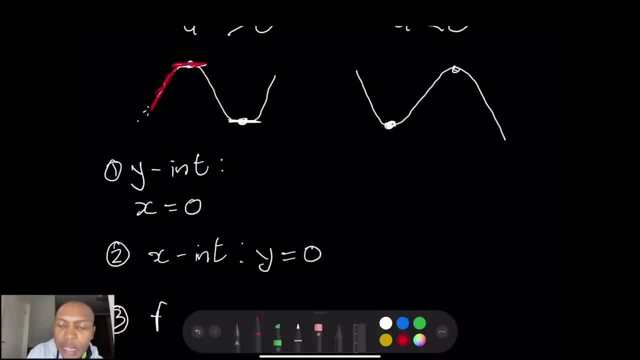 but it keeps decreasing until it gets to that point there where it becomes zero. and then what happens? your gradient now starts becoming negative there, and in this case until it becomes zero over there. so you know, every time at your turning point it means that this is where our gradient, and how do we get the? 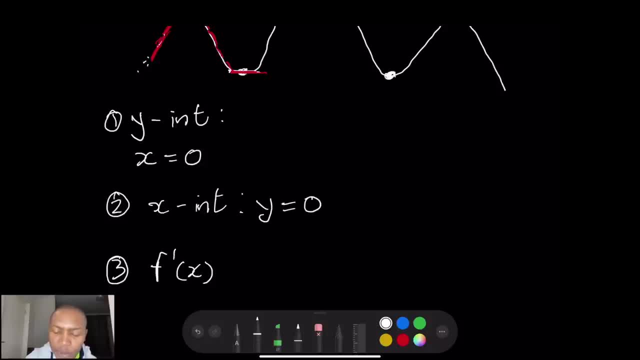 gradient. we take f, prime x, f, dash x, the derivative, and we make that equal to zero. so we know, at the turning point we make the gradient equal to zero, okay, and the derivative rather equal to zero. and how do we find the y value of the turning point? so in this case, we'll just substitute the. 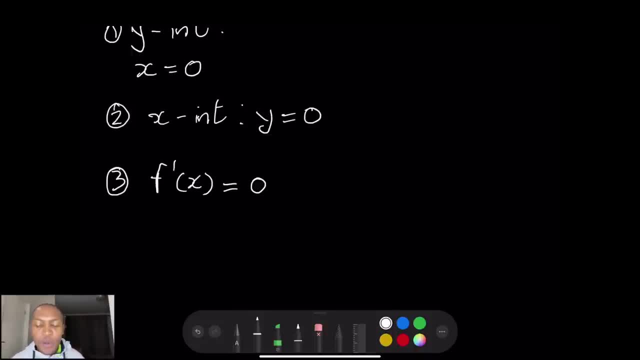 x value back into the equation. okay, right now. so we know this is, this is how we get our turning point. okay, so the x value of your turning point and, of course, your y value of your turning point. you'll take whatever value of x- let me say x turning point- and you're going to substitute: 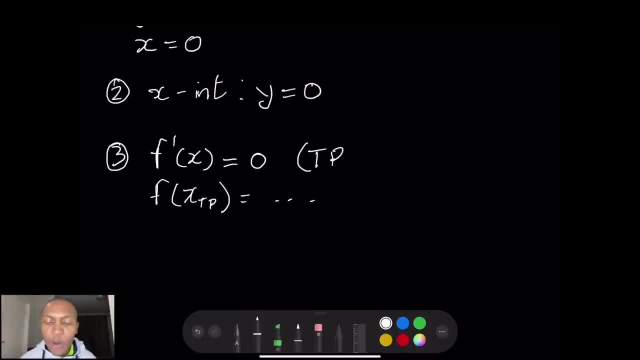 it back into your original equation. all right, so we know that the derivative equal to zero gives us our turning point, or our maximum and minimum values. right, and then number four. right now, please, i want you to listen carefully on this one. we call it a point of inflection. 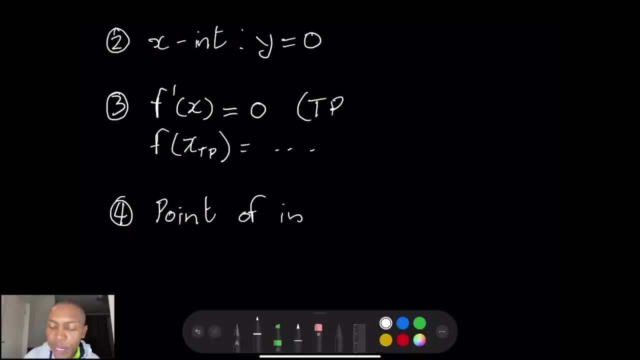 okay, so call it the point of inflection. i'm going to explain just now. so the inflection point: this is what differentiates your graph from being you what we call a concave up shape and a concave down. now, at the point of inflection. 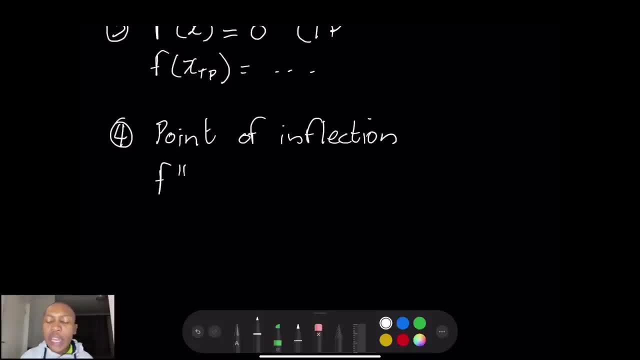 we say that, well, the you take the derivative of the derivative. so it means that at the point of inflection you take the double derivative and you make it equal to zero. okay, and the x value that you get there is what we call the point of inflection. now suppose we say: okay, we get the. 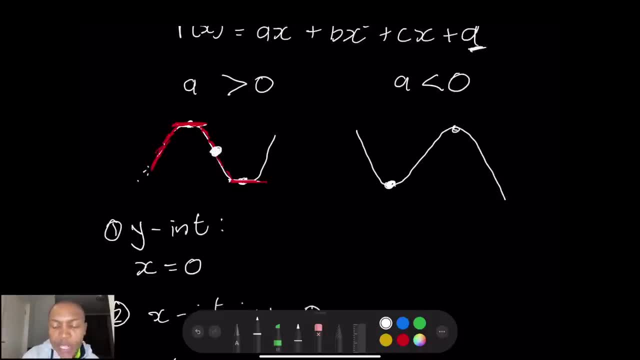 point of inflection. and that is your point of inflection, right? so it means, before the point of inflection, your graph. let me talk about this one in particular. where a is greater than zero, it means that our graph is a. in this case, it's going to be a concave down shape, can you see? 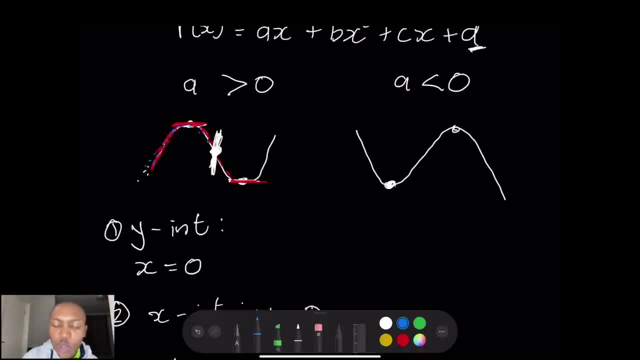 so it's almost like you know that blue color. so it shows you that it's a concave down shape, right? so after the point of inflection, then what happens is that it becomes a concave up shape. so what differentiates between the two points or the two parts of your graph where it becomes concave up? 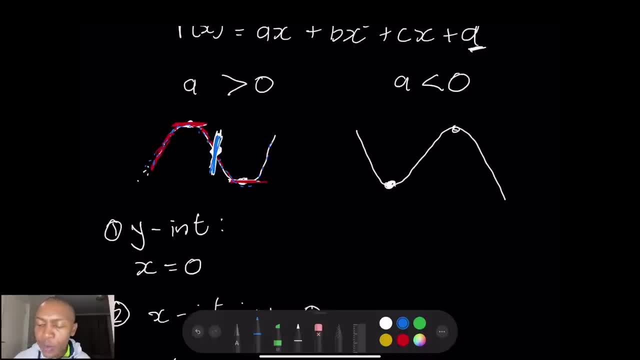 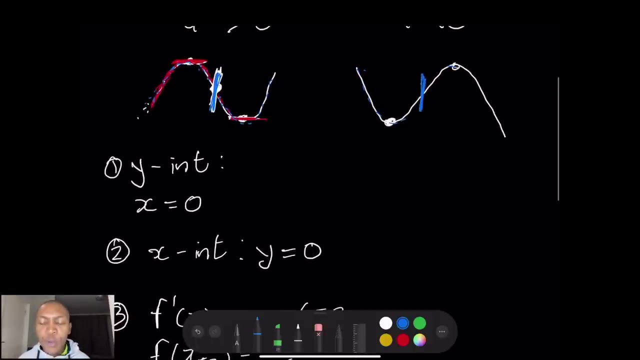 and concave down. that is your point of inflection, all right, and of course, even on this graph over here. okay, if we get the point of inflection, so here it starts by being a concave up and and a concave down. now just a couple of things for you to remember. okay, so now we know that to get the 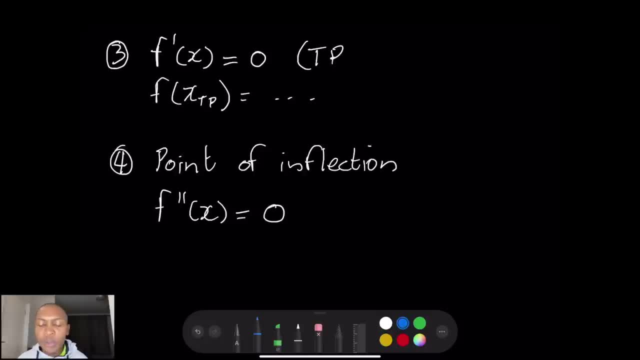 point of inflection, we say, well, this is where the double derivative is great, i mean is equal to zero. but what does it mean when the point of inflection, let's say, you get the point of at the, you get the point of inflection, and you get the point of inflection, and you get the point of inflection. 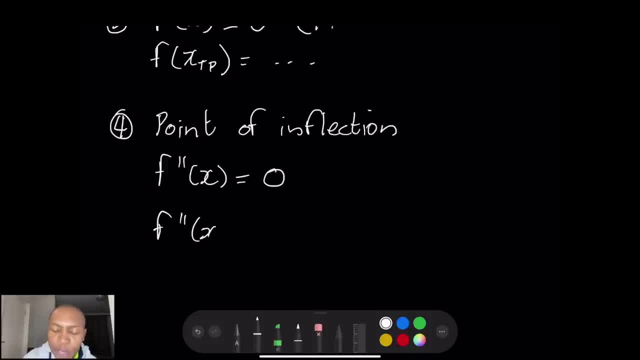 you know a particular point, often a particular point. you take the double derivative. what does it mean? when you say: well, the double derivative, you get it to be greater than zero, right? so all it simply means: when the double derivative is greater than zero, it means, in this case, you are. 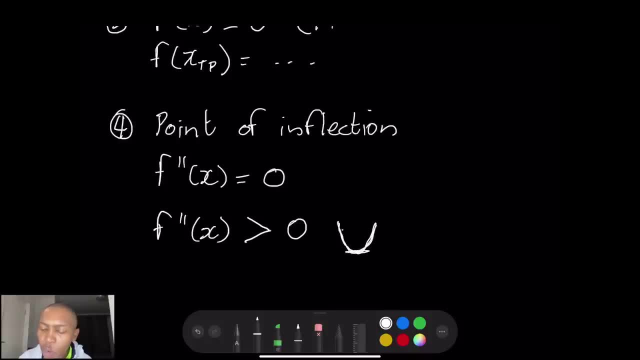 dealing with a minimum, a local minimum, okay, and so you are dealing with a concave up shape, but where the double derivative is less than zero. please just remember this, okay. so in that case you are where it's less than zero. you are dealing with a that concave down shape in that case. so 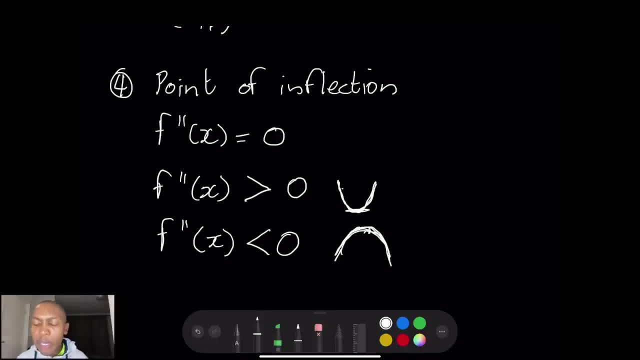 it means that you are, you would be looking at a maximum, okay, between those points. right, and we're going to apply this when it comes to graphs. okay, in this case. just another thing to just remember is that, remember, when we are talking about the point of inflection, okay, we said, this is where. 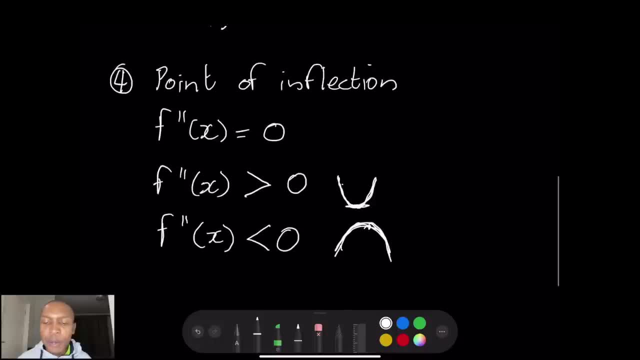 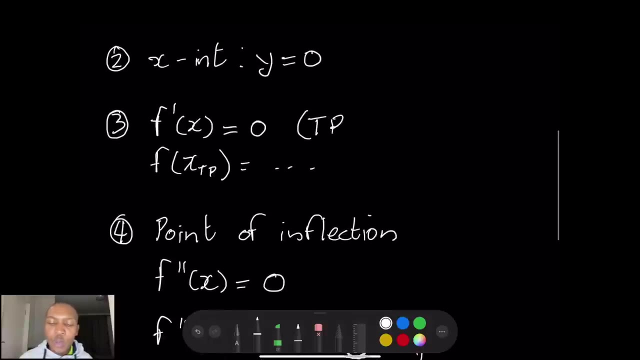 the graph, we differentiate between the the different points. all right, where you've got a local maximum and a minimum, all right. where you've got a concave up- okay shape- and a concave down, all right. and in this case, right. going right back to your derivative. remember when you are talking about the derivative. now i want 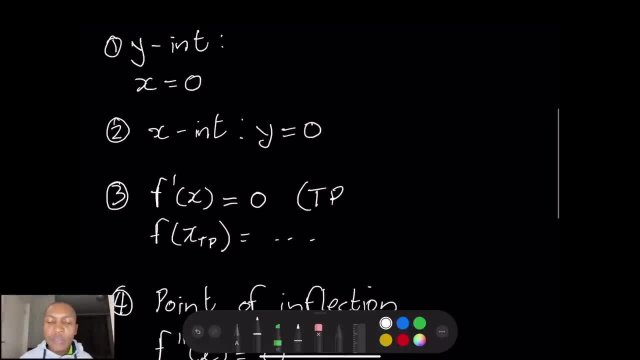 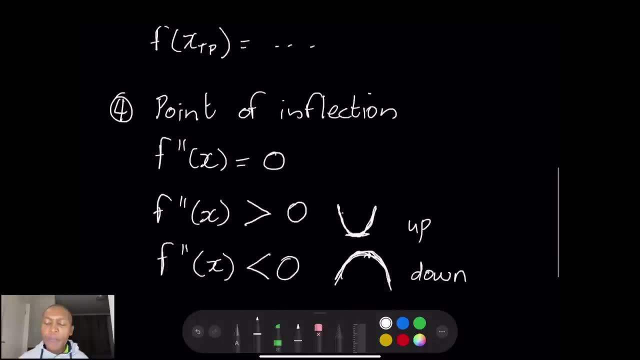 you to just stay a little bit on this one. when we're talking about the derivative, you are talking simply about, in this case, the gradient of the graph. now i'll just quickly take an example. okay, if i draw a graph that looks like that, okay, let's just take a shape. all right, now there's a difference. 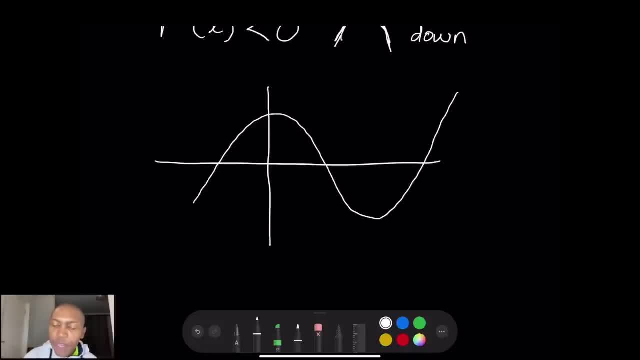 between f of x. okay, let's say: what is the difference between f of 4 and f dash of 4, right? so this is the y value at x's is equal to 4. now look at this. if I were to say this is at x is equal to 4, right now, what happens? 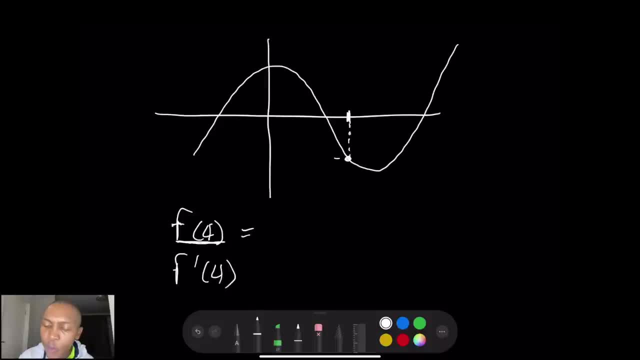 I would find there is my y value where x is equal to 4. so here, if I say that value is 4, the y, the corresponding y value is f at 4. so in this case you'd say this is 4 and f at 4, right? 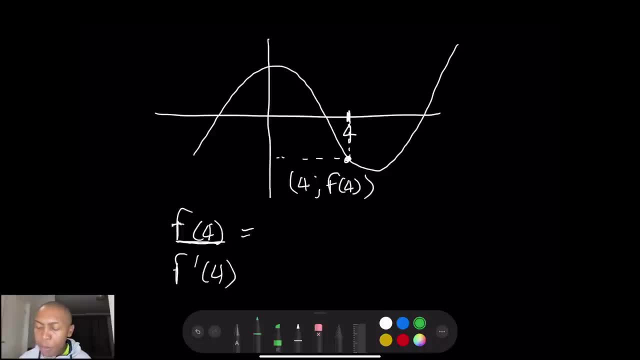 but when you say f dash at 4- now I'm going to indicate this in a green color- right, you are simply saying what is the gradient? all right, where x is equal to 4, right, f dash at 4. so you'll see that that gradient over there is negative. okay, right. 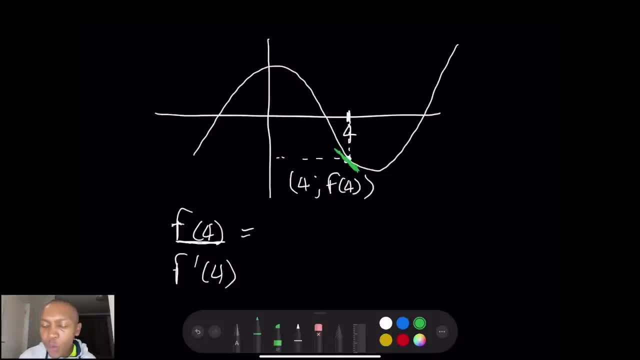 now there's a difference, in this case the y value. okay, you'll you'd find that your y value is equal to 4, so you'll see that that gradient over there is negative. okay, right now there's a also negative there, but your gradient is negative. but let's say you take another point. 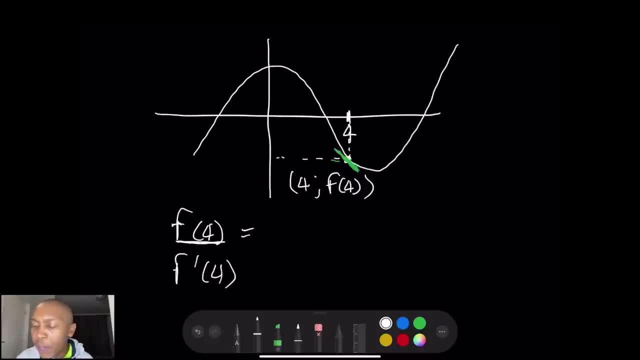 okay, and I'm deliberately going to pick a point here, right? so let's say we pick a point over there. let's just say, just for argument's sake, it's where x is equal to 7. now, in this particular case, you can see once again, if I pick a point there once again, you'll see that your f 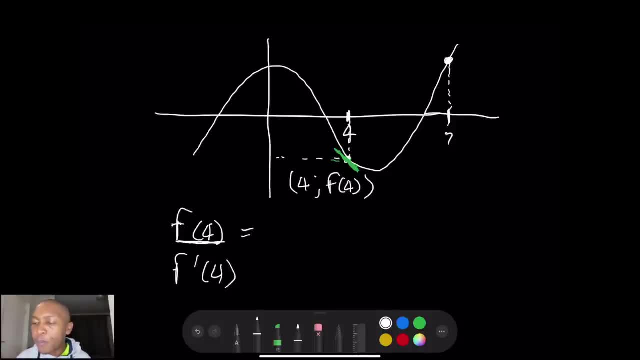 of 7 is a positive value, but also look at that your gradient at this point is also a positive. you know the right hand tick right, so your gradient is also 7. in this, I mean your, your gradient is also positive. okay, but look at where I get you know, I'm going to make this at this particular 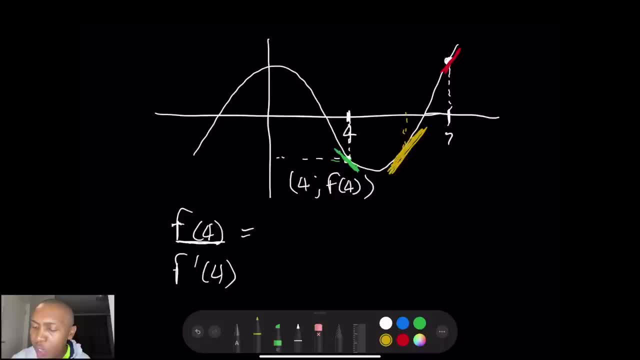 point. okay. so what happens? your gradient is positive, but your x value, I mean your y, your corresponding y value at that point would be a negative value. It's on the negative axes, right Y values. right Now, in this particular case, you must be able to. 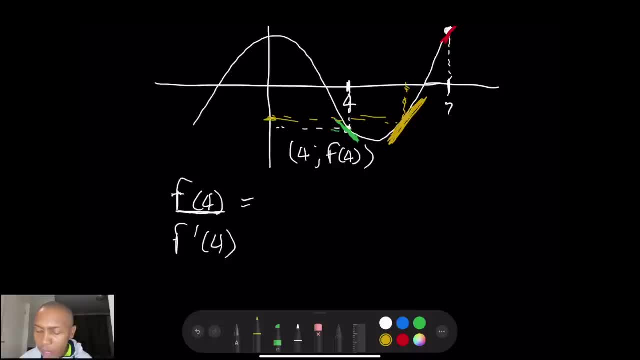 tell the distinction between the gradient. okay, Now notice this. If I were to talk about the gradient here, okay, let me just indicate it. So in this particular case, your gradient is positive, positive, positive, positive, positive until it becomes zero. over that point, Then look at this: 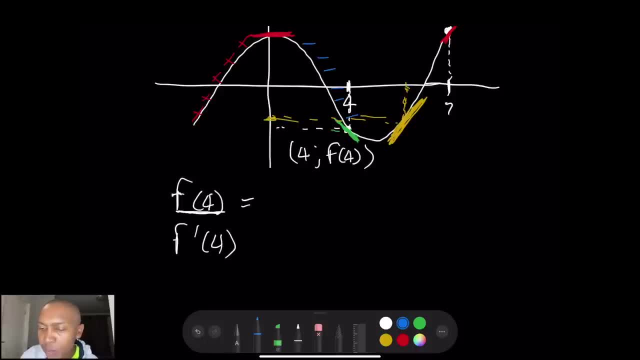 your gradient therefore becomes negative, negative, negative, negative, negative, negative, negative, until it becomes zero. at that point, right, And then it starts increasing again, it starts becoming positive. But look your y values right, I'm going to indicate them in green. They are negative, negative, negative. 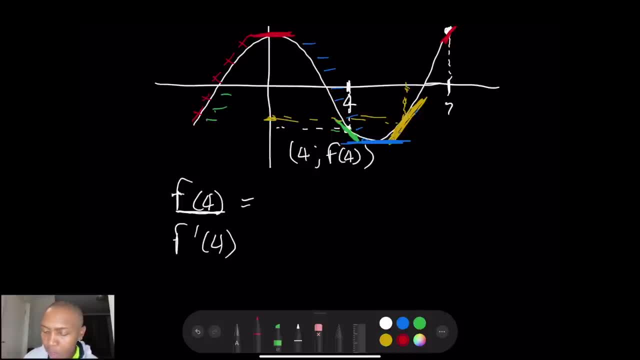 and when you get over that point, okay, let me just indicate them in white so they become positive thereafter. So you must be able to make a distinction between when we're talking about the y values as well as when we are talking about, in this particular case, the gradient of the graph. 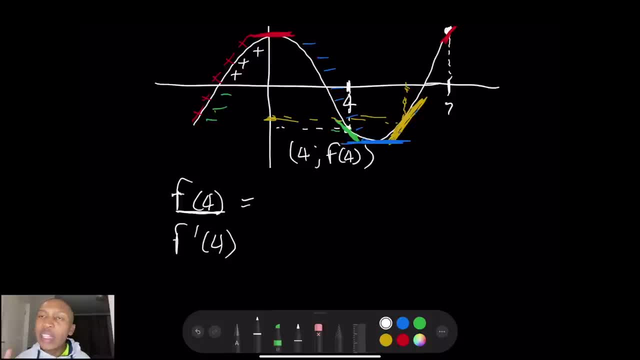 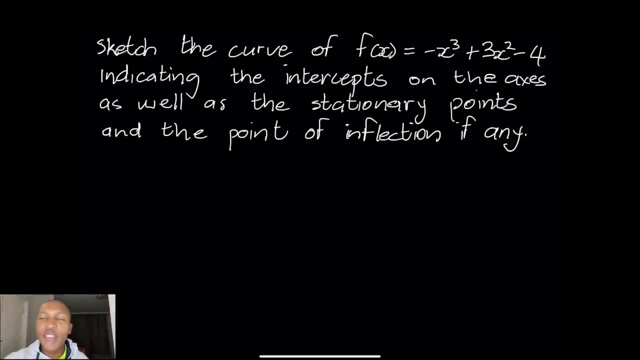 okay, I think we've done enough. All right, let's get into an example of how we are going to apply this. All right, let's take our very first example. All right, so they say: sketch the curve of f of x. 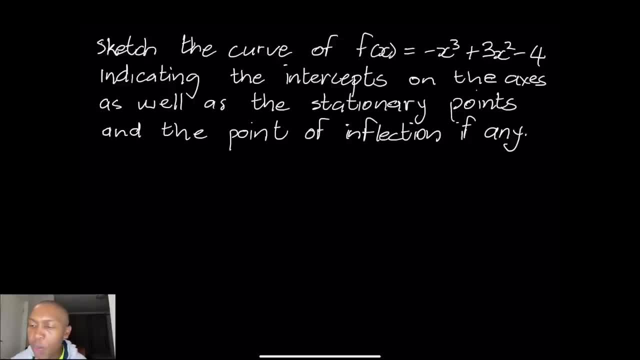 is equal to minus x cubed plus 3x squared, minus 4.. And we're going to indicate all our intercepts on the axes, as well as the stationary points Now talking about that word, stationary points. so in this case, we're going to apply this. So we're going to apply this, So we're going to 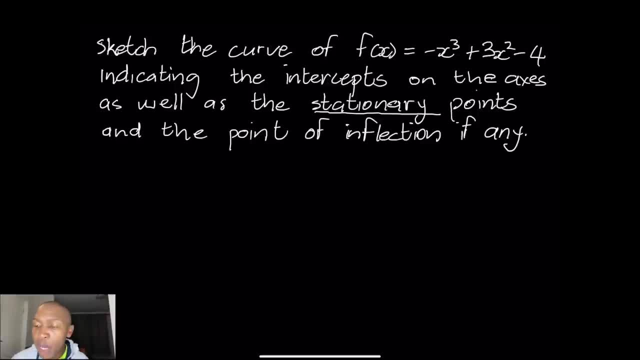 our turning points or our minimum and maximum values are also called stationary points. Please remember that right. And they say: also indicate the point of inflection. if there is any right Now, let's first of all start with what we usually do, just the normal stuff. So let's find the x. 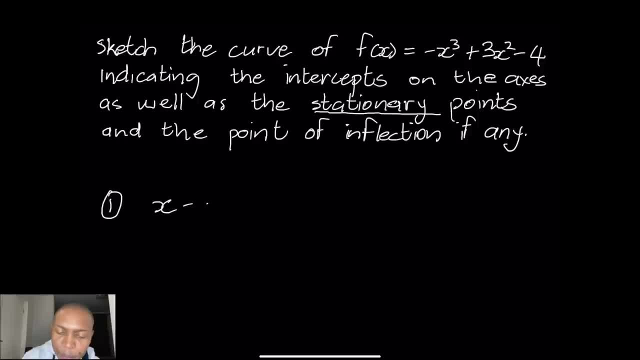 intercept. So we're going to say: well, what happens at the x intercept? Oh, first of all, before we even get to the x intercept, what are we expecting when it comes to this graph? okay, We're expecting. 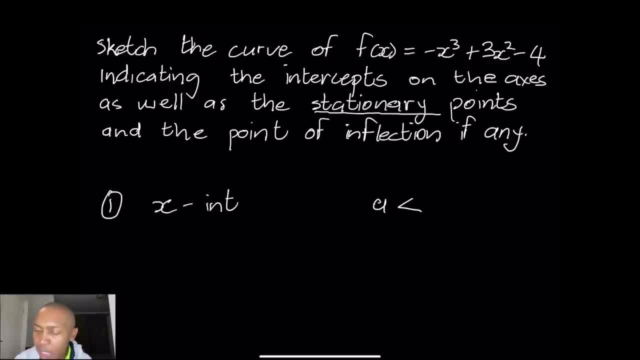 because the value of a in this particular case is less than zero. So I'm expecting a graph. ultimately, that would look like this: okay, So the shape of the graph should look more or less like this: Like that shape over there. all right, So we're going to start with our x intercept. okay, So. 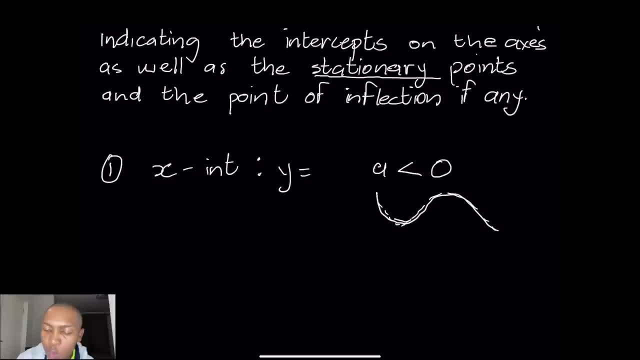 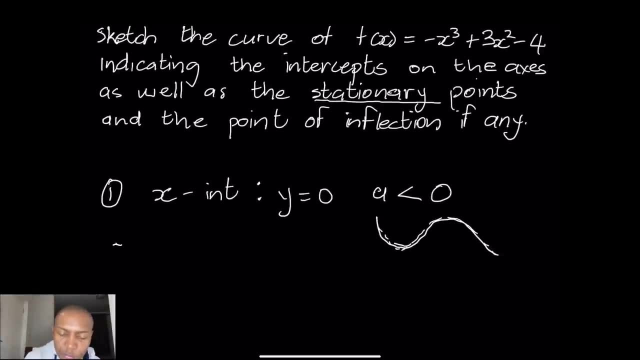 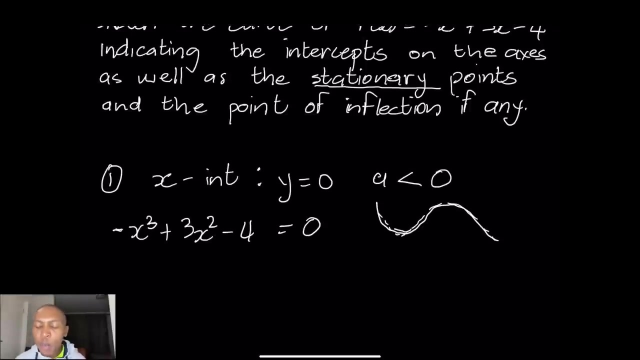 we said what happens at the x intercept. we know this is where y is simply equal to zero. okay, So remember so. then we take minus x cubed, okay, plus 3x squared, minus 4, and we know this is equal to zero. Now, remember what we said, ladies and gents, in our previous. 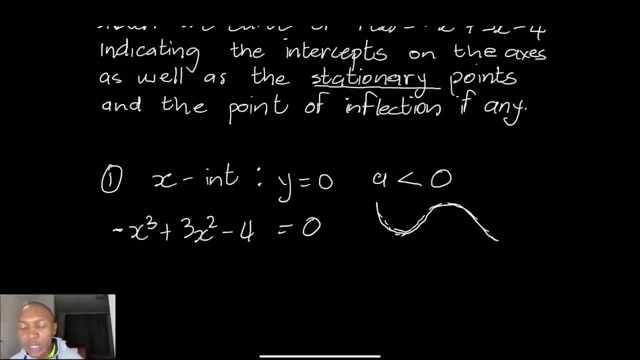 videos, how do we factorize a cubic function? or all we simply do? in this case, we're going to look at for one of the factors right, So let's see. So what can we substitute? first of all, 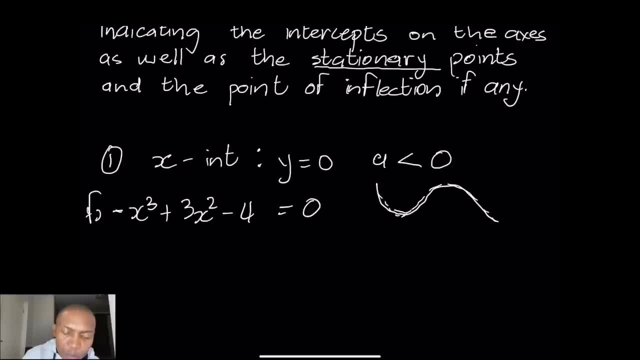 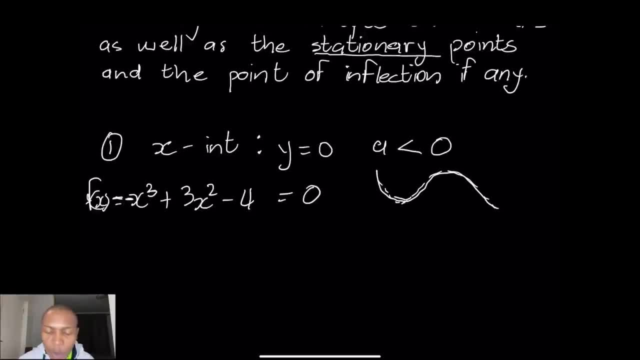 okay and all of that. So now let's substitute. let's say first of all f of 1. Let's see if that works. So that's going to be minus 1.. So everywhere I see x cubed rather plus 3 times. 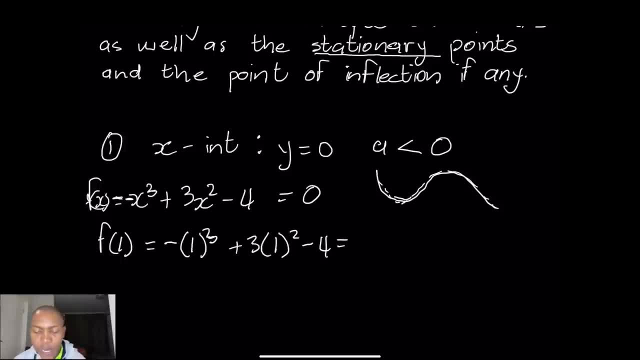 1 squared minus 4.. Let's see if that gives us zero. Okay, So that's going to give us minus 1, squared minus 3, minus 4.. And definitely that does not give us zero. Okay, So we end up with. 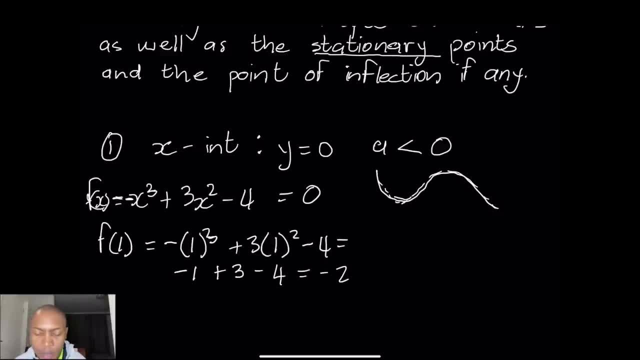 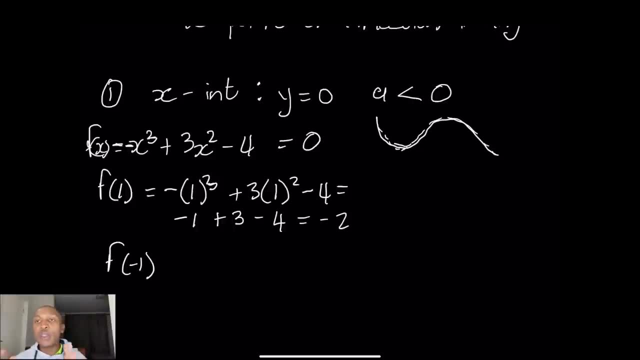 actually minus 2 in that case, right? So that doesn't work. So let's try f of minus 1.. Okay, So remember, we said: you try 1, then minus 1.. You try 2, then minus 2, until you get a value. 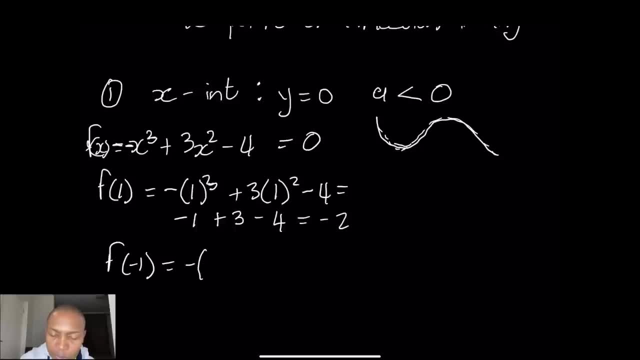 that will give you zero. So I'm going to say, well, that's minus a negative. So where I see x, I'm going to put negative 1.. Okay, Plus 3 times negative 1 squared minus 4.. And let's see what that gives us. So I've got minus a negative 1.. So that becomes: 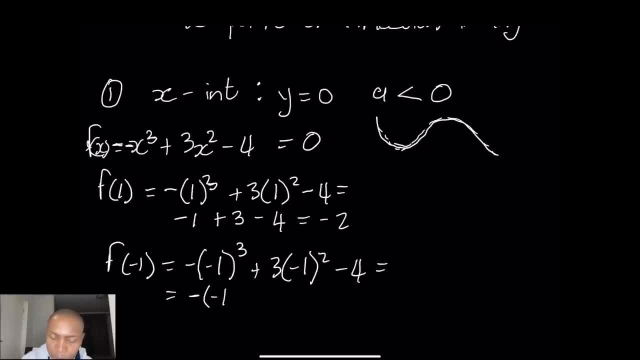 a positive 1, because that's going to be minus a negative 1 plus a negative 1, squared is 1.. So that's going to be plus 3 minus 4.. And in this case, if I look at this, negative times a. 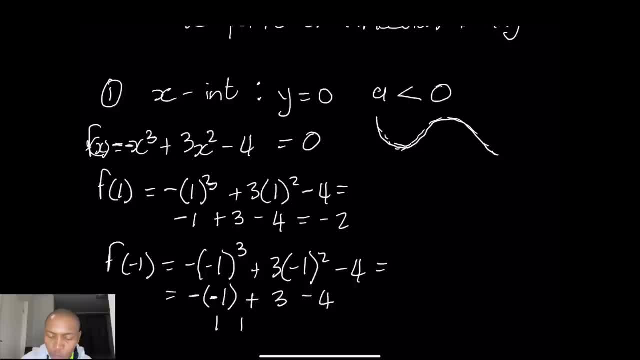 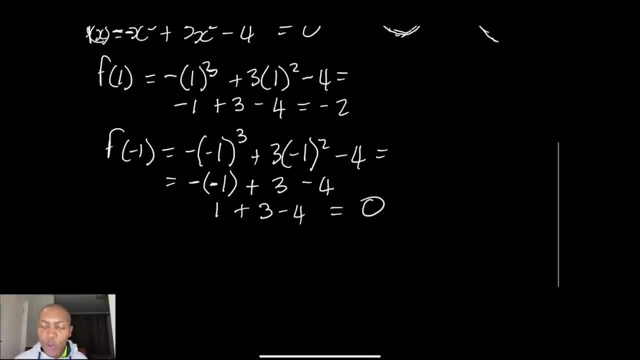 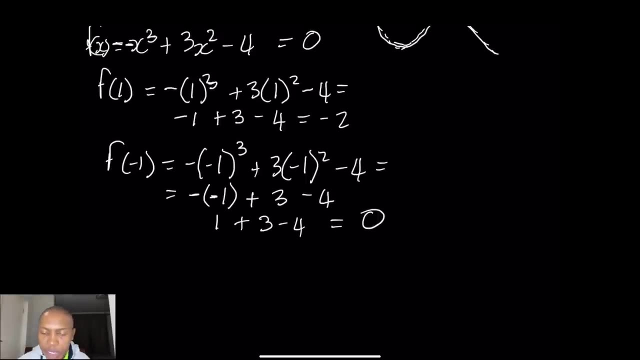 negative will give me a positive, So that will be 1 plus 3 minus 4.. And definitely that gives me zero, Okay, So now I've got one of my factors. Okay, So one of my factors is actually x plus. 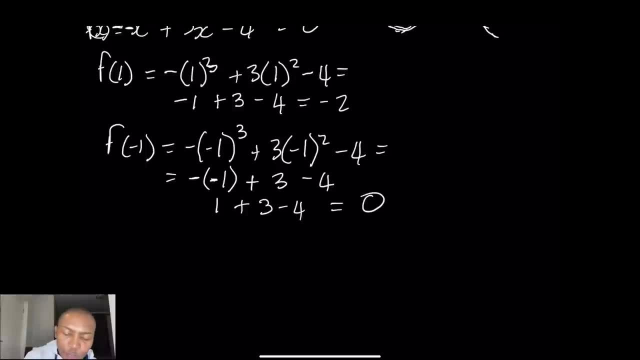 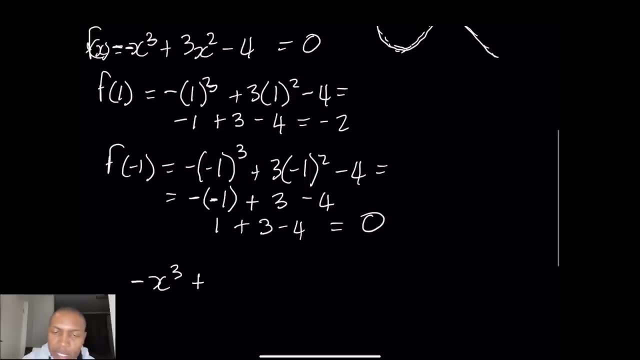 x plus 1.. Yes, Correct. So this is going to give me a positive 1. So that's going to be negative 1. So I'm going to now say: well, it means that minus x cubed, plus 3x squared, minus 4. 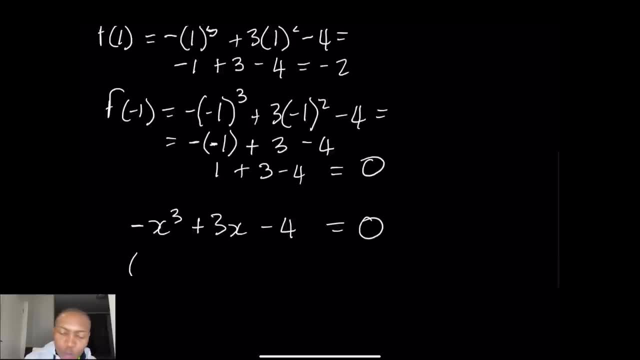 is equal to zero. But we already know that x plus 1 is a factor. But you know what I'll do, In fact? let me do this: Let me just multiply everything by a negative, in this case, so that I have negative 1.. So I'm going to now say: well, it means that minus x cubed, plus 3x squared. 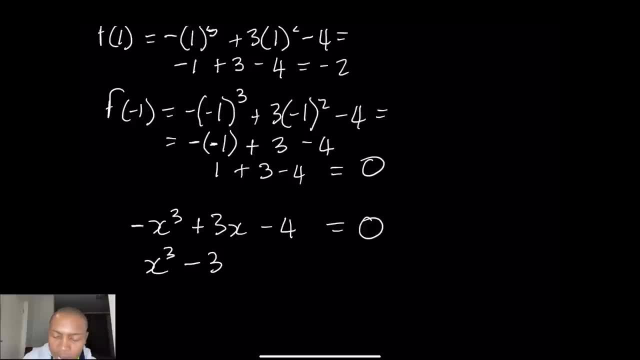 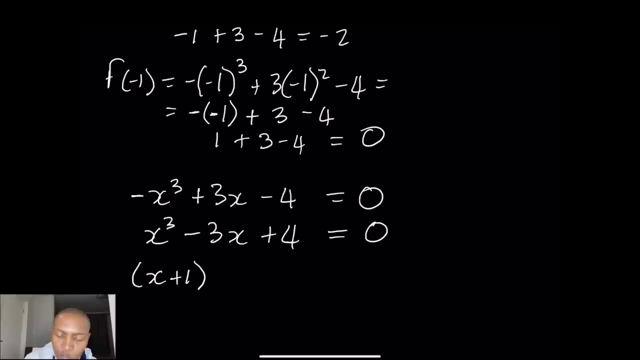 minus 3x plus 4.. So when I multiply by negative, it changes sign. Remember: negative 1 times zero would still give me zero. Okay, So I know that x plus 1 is one of the factors. Now let's find. 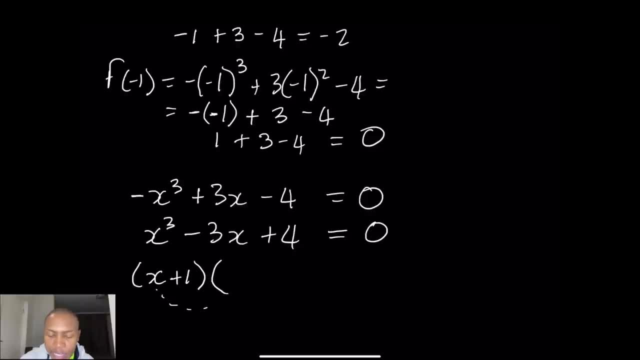 the other factors Right. So now? negative 1 multiplied by what will give me x cubed, That will give me x squared. Okay, Let's go to the last one: Negative 1 multiplied by what will give me positive 4.. Or rather: 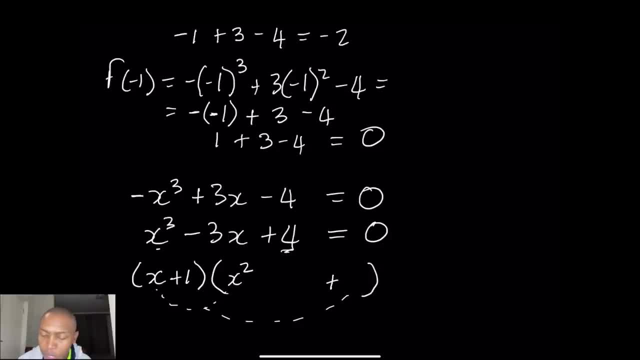 1 multiplied by what will give me 4.. That will be plus 4 there. Okay, So that I get that last term. But in this case, oh, I left a square there, Sorry about that. Okay, So now I need to find. 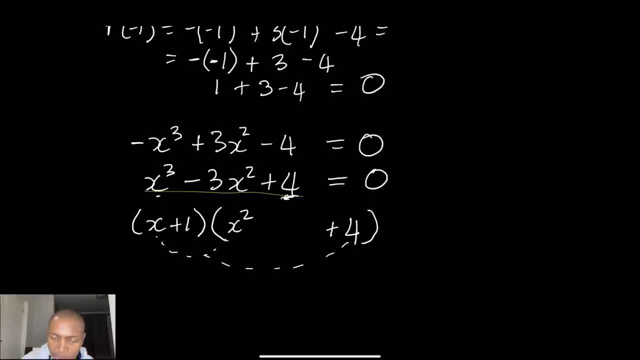 the middle term over here, Right? So I will say: well, in this case, what will I do? Well, negative 1 times x squared will give me positive x squared, Right, Okay, Let me just remove this so that it's not confusing. Okay, So let me do that in the yellow. 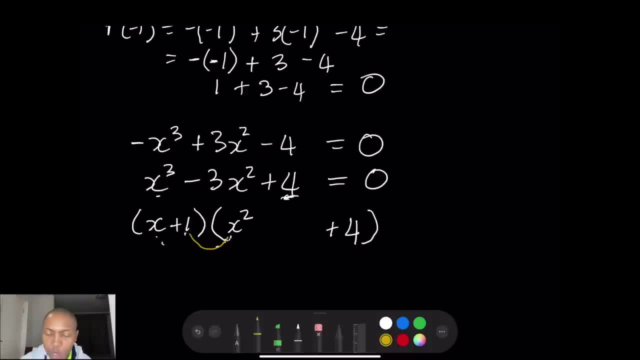 in fact. So negative 1 times x squared will give me x squared, X squared Right, But I want to have 3x squared ultimately, right. so in this case, x multiplied by what? okay, in this case i want to have, ultimately, the result should be minus 3x squared. so, in this case, what do i need to add to? 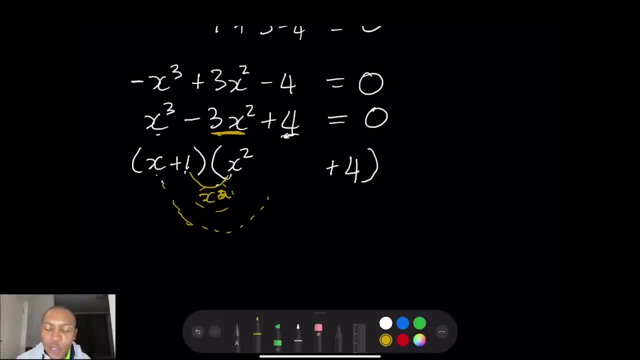 the x squared in order to get minus 3x squared, and you'll see that i will actually need minus 4x squared in this case. so minus 4x squared plus x squared will give me 3x squared, do you agree? so we already have this from that, isn't it? so how do i make minus 4x squared? so x multiplied by what? 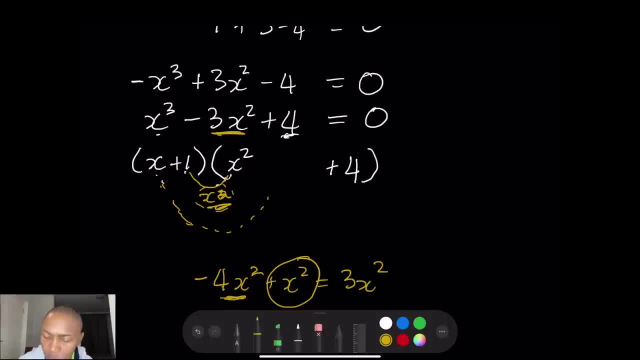 will give me minus 4x squared and you'll see that that will be minus 4x. so that will be minus 4x squared. so that will be minus 4x squared. so x multiplied by what will give me minus 4x. so that when I multiply this into that, I get x squared. when I multiply that into that, I get 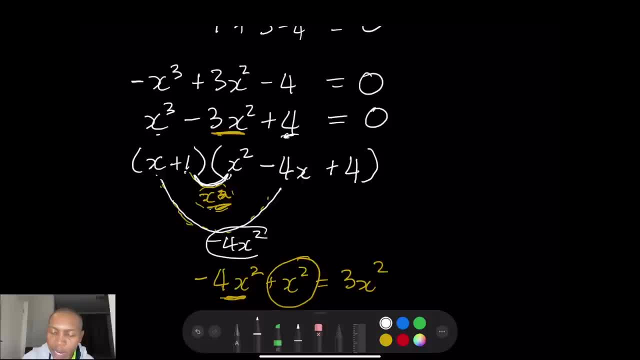 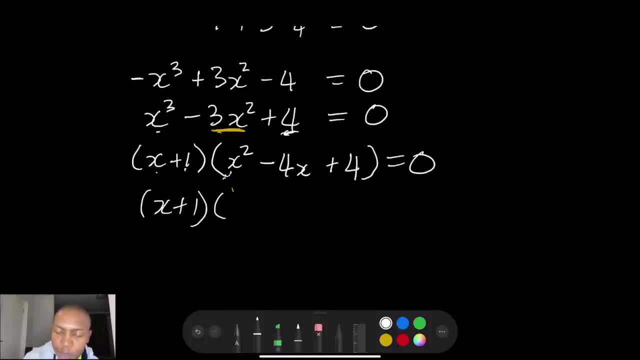 minus 4x squared, and when I add this to that, I get minus 3x squared. I hope that makes sense, ladies and gents. okay, right, so I've got my other factor. and now? so this will be equal to zero. okay, so that will be equal to zero, and you'll see. so I've got x plus one into now if I factorize. 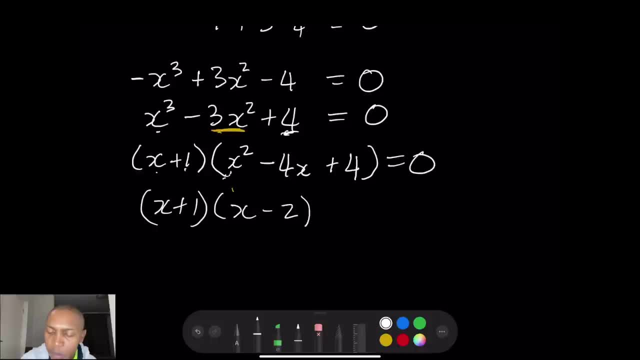 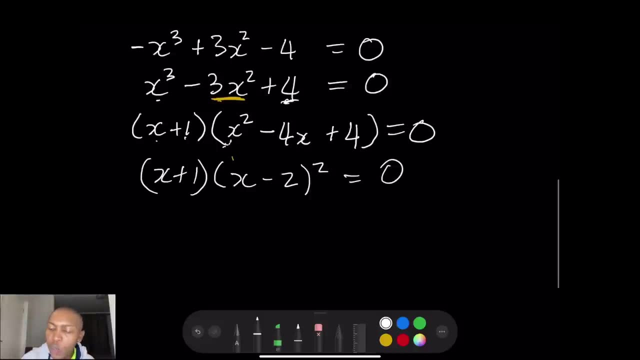 that I can see. this is going to give us x minus two squared right, so this will be x minus two squared right. so this will be x minus two squared right. so this will be x 2, x minus 2. so essentially, we know that our x intercept is: x is equal to negative 1 or x is. 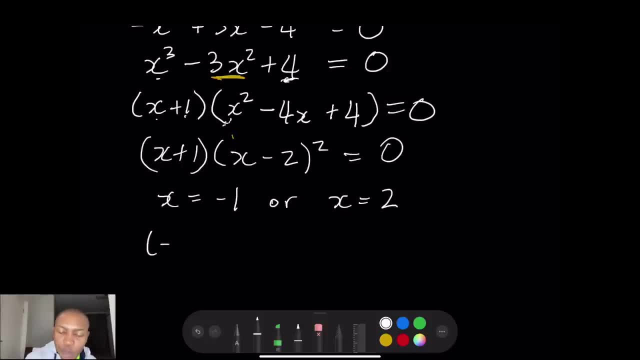 equal to 2, so it means that our x intercept will be at negative 1 and 0, and okay, it will also be at 2 and 0. okay, so those are our x intercepts. now let's go to the y intercept. so we said we'd look. 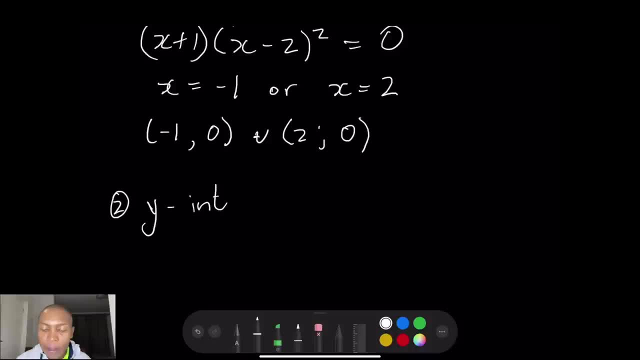 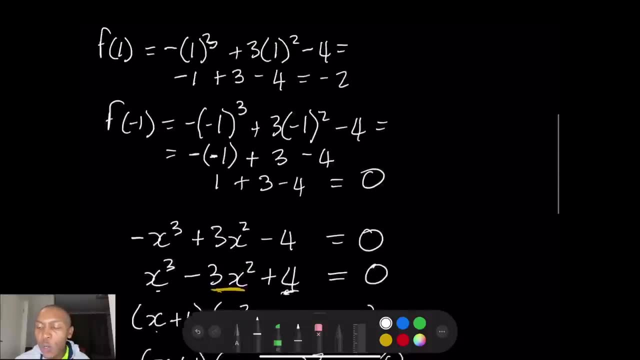 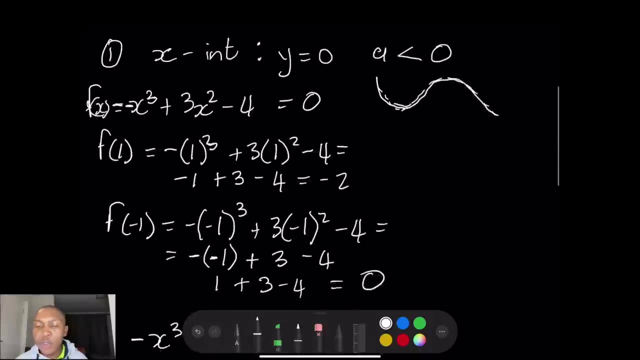 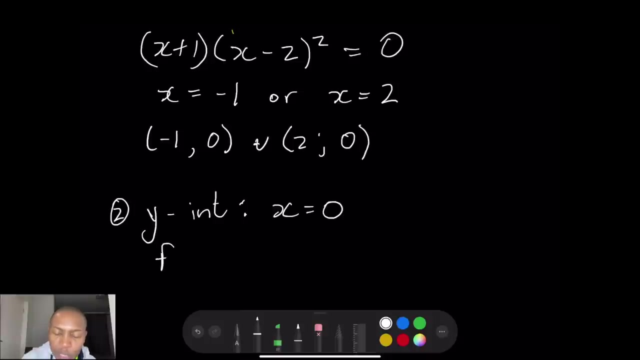 for the y intercept. remember, we're moving swiftly towards getting that graph. so this is where x is equal to 0 and, of course, if you've got your equation in standard form, right, remember we said that constant value there always gives you your y intercept. so, So, without necessarily going into, okay, so in this case we say f of 0. this is going to be. 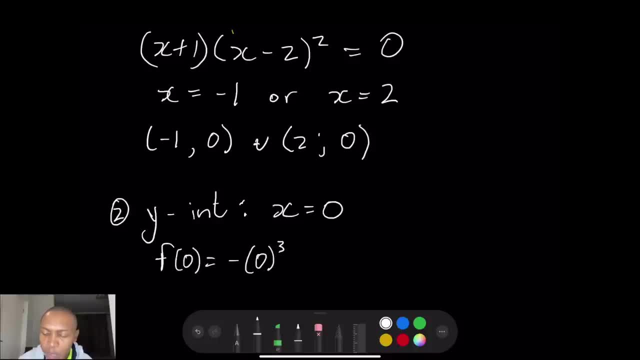 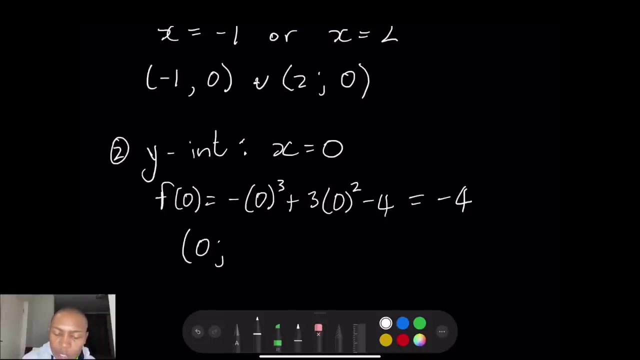 minus 0 cubed. okay, that was remember. that's plus 3 times 0. okay, so that's plus 3 times 0 squared and that's minus 4, and you'll see that that gives us simply minus 4. so our y intercept is: where x is equal to 0 and y is negative 4. 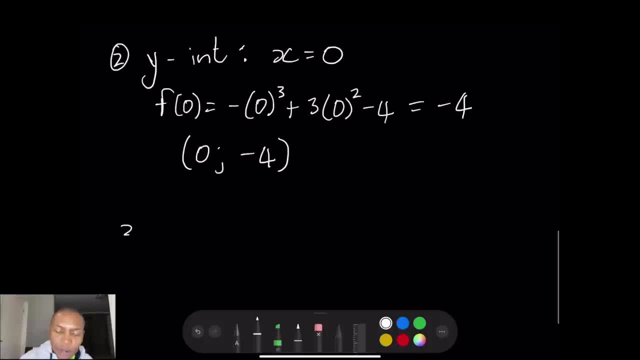 okay now, um, we're looking for our stationary points, or what we call our turning points, right? so how do we get the turning point? remember that f of x, okay? okay, let's write down the equation. so that's minus x cubed plus 3x squared, minus 4, right? so that's our equation. so how do we get the turning point? we? 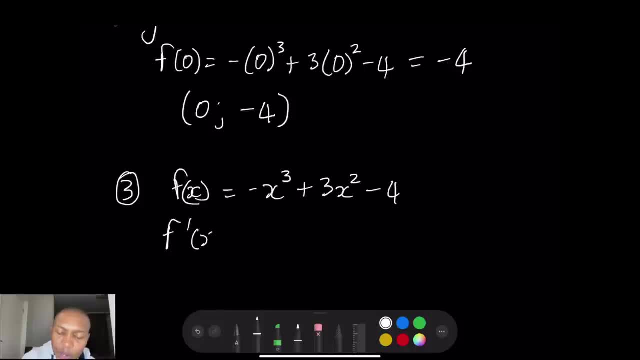 said, the turning point is where f prime x, which means the derivative is equal to zero. so let's find our derivative there. so our derivative, we said, jump down, that's minus 3x squared plus 6x. okay, that's a constant. so that will be zero, and so this is equal to zero. so now, 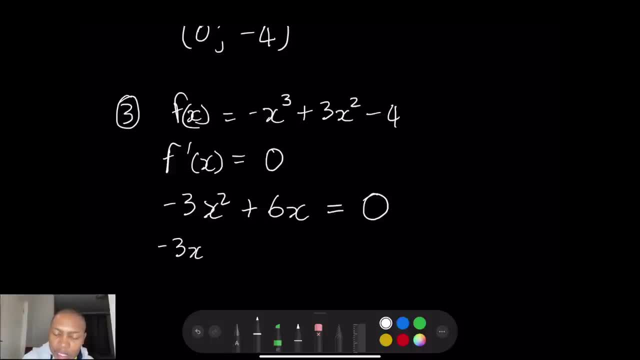 let's find our value. if i take out minus 3x as a common factor, so that will be x minus 2, this will be equal to zero. so it means we've got a stationary point where x is equal to zero x. we've got a stationary point where x is equal to two. okay, and how do i get the y value of my? 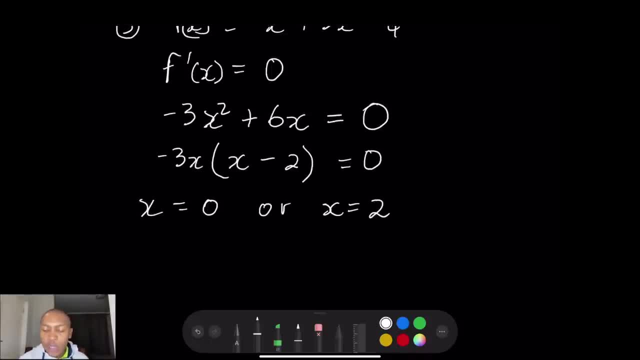 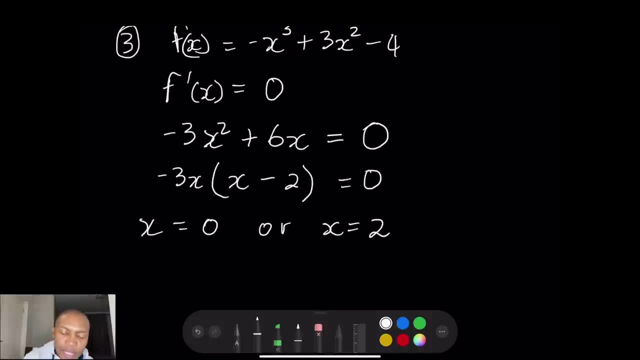 stationary points. all i simply do is to take the x value and substitute it back into the original equation. please remember that. so remember, i already have f of zero. okay, right, if you substitute, that will give you minus four, so which means zero, and minus four is equal to zero, so that's. 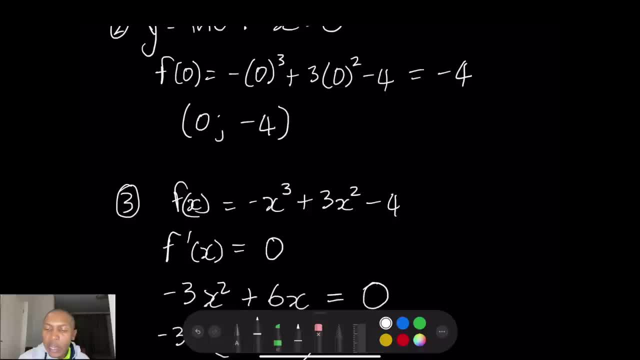 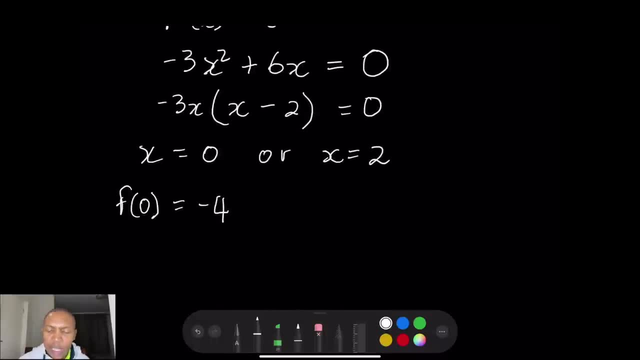 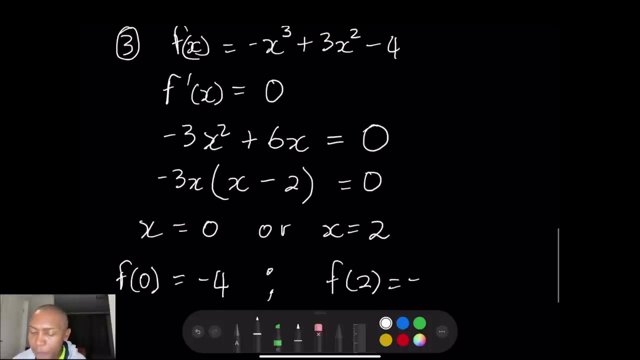 four is not just a y intercept, but it is also a turning point. okay, i hope you can get the. you know just the picture there, okay. and then also it means that f of two, now let's find f of two. in this case, this will simply give us minus two cubed, plus three squared, plus four plus five squared. 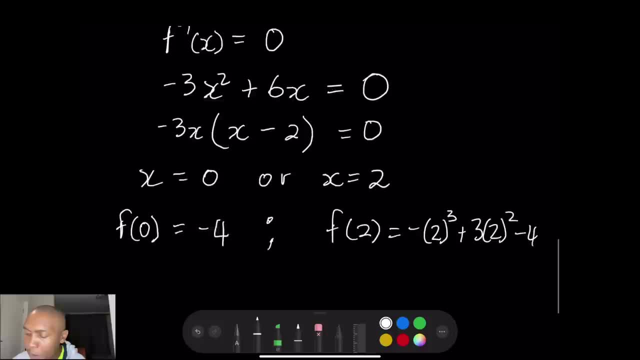 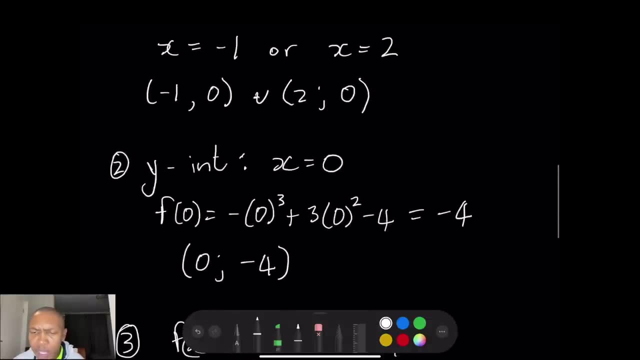 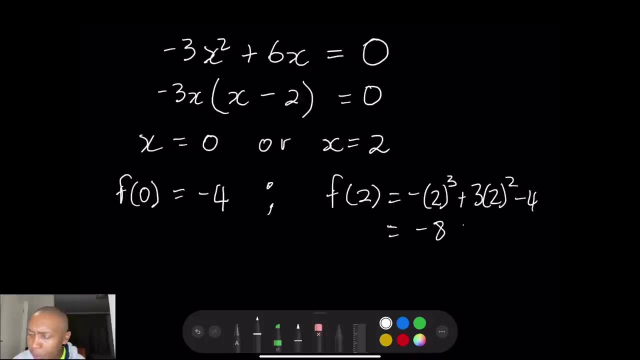 times 2 squared minus 4. okay, and in fact I think we had found X, so that's 2 and 0, right? yeah, it should actually be so that would be minus 8, plus, in this case, 3 times 2 squared, that's 12 minus 4, and yes, and it does give us 0 there. so in 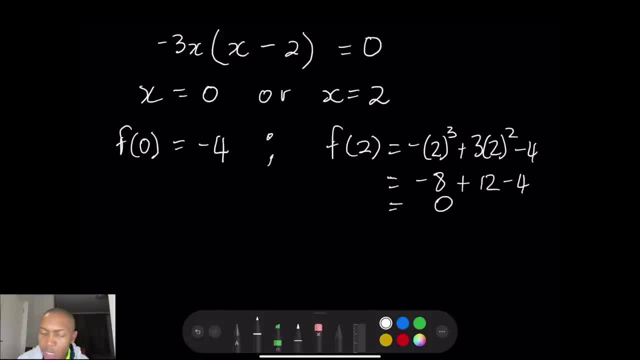 this case we also have 2 and 0 as a turning point, so in this case it means that our turning point will be at 0 and minus 4. okay, but it also means it's going to be. we've got another one which is at 2, where X is equal to 2 and Y is. 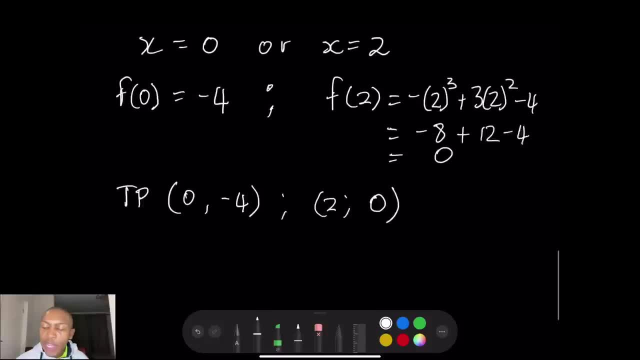 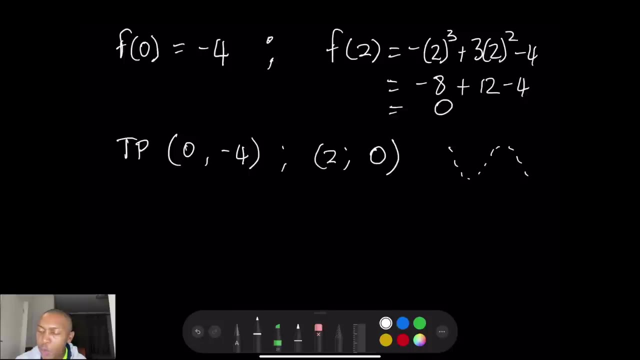 0 as well. alright, so of course we can also find the point of inflection. so I hope you can more or less see the shape of the graph, because, remember, the a value was negative in this case, so it would be a graph that actually looks more or less. 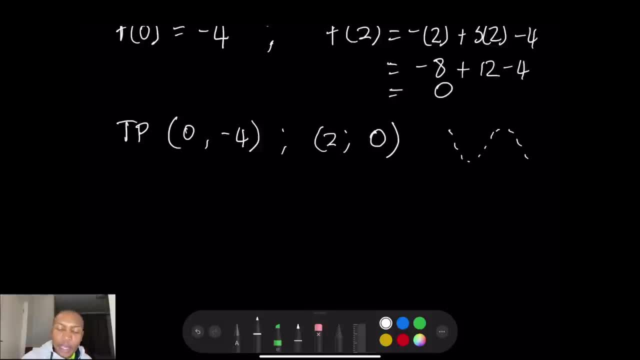 like this: okay, right, so now our point of inflection. so we said what happens at the point of inflection? okay, so inflection point. right, so our inflection point. you'll see that we say: this is where the F, you know, F double dash of X is equal to 0. so, which means I'm taking the derivative of the. 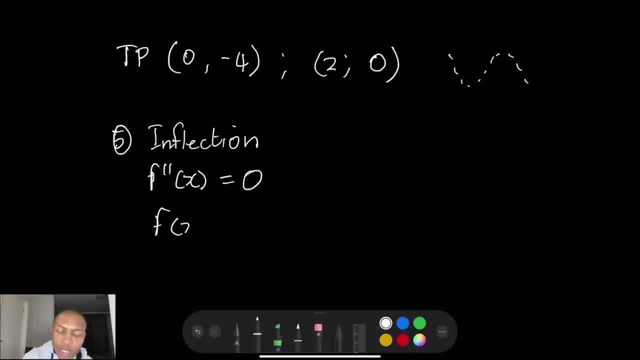 derivative. now remember what was. okay. let me start with F of X. F of X was minus X, cubed plus 3x3 squared minus 4, right, but what was F dash X? that was minus 3x squared plus 6x, right, but what's the? 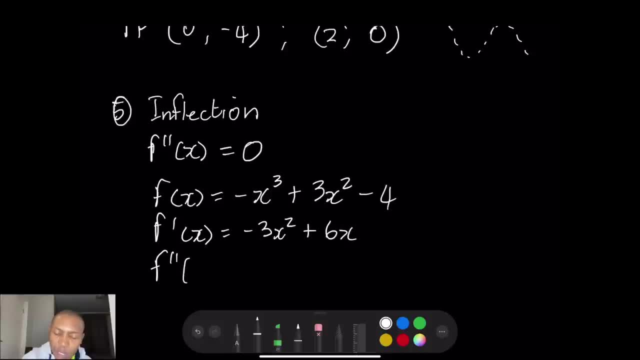 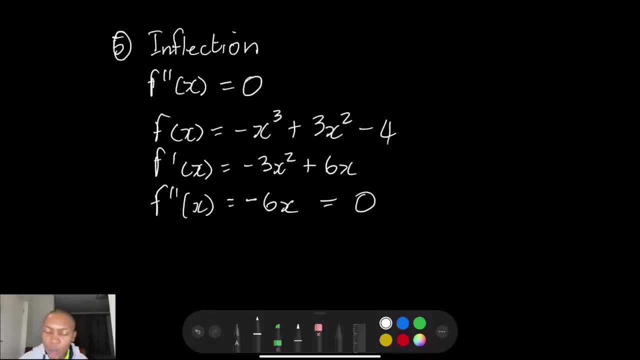 double derivative. in this case that's going to be F dash, double dash of X, which is going to be minus 6x. and we know that at the inflection point, this is where the double derivative is equal to 0. and so what does that mean? it means 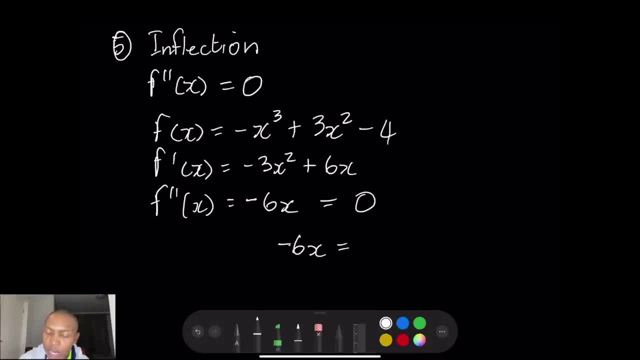 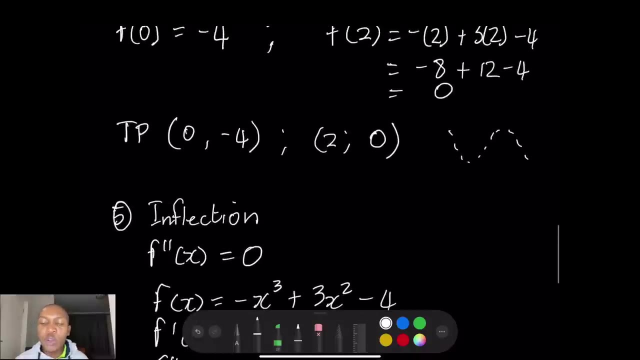 that again, if I say minus 6x is equal to 0, it means dividing both sides by negative 6. therefore X would be equal to 0. so it means our inflection point will be at X is equal to 0 and of course we already know where X is equal to 0. Y is. 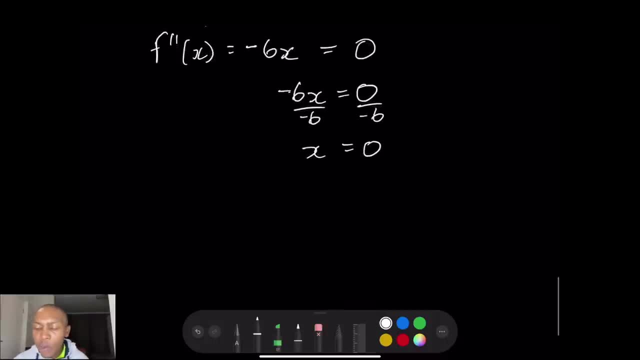 minus 4. okay, right now, ladies and gentlemen, I think we are almost ready to draw a graph. okay, so what does our graph look like? and, of course, this will not be an attempt to draw an accurate graph, it's just to give a picture of what our 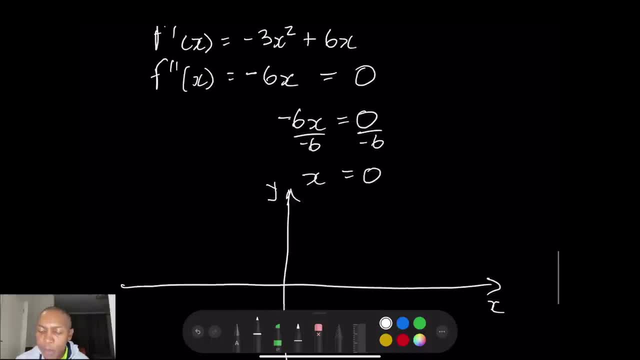 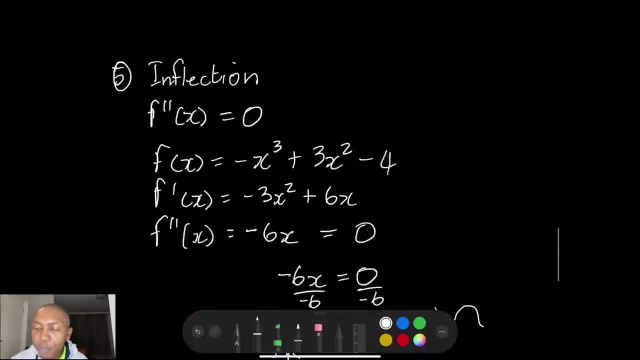 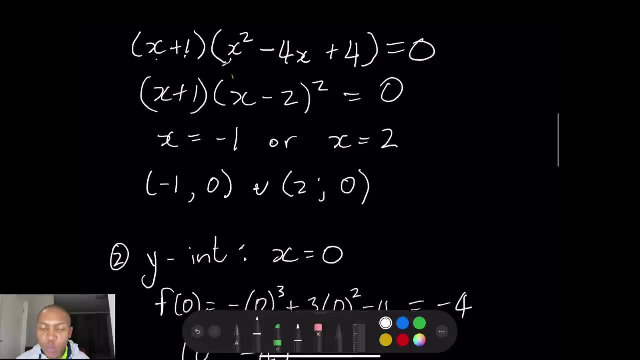 graph looks like. okay, so we know what the shape should more or less look like. we said we are expecting a shape that looks like this. so first of all, we set our X intercept. okay, remember, our X intercept was at minus 1 and 0. okay, so we know. 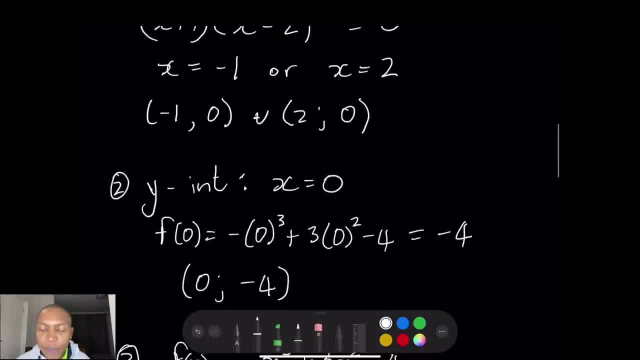 that we're going to cut where X is minus 1 and 0, and we know that we're also going to cut it two and zero, right? so, uh, minus one and zero. so there's our minus one there. so that's our first uh intercept there, and then, uh, we're going to also have at two. uh, okay, maybe let's leave a little. 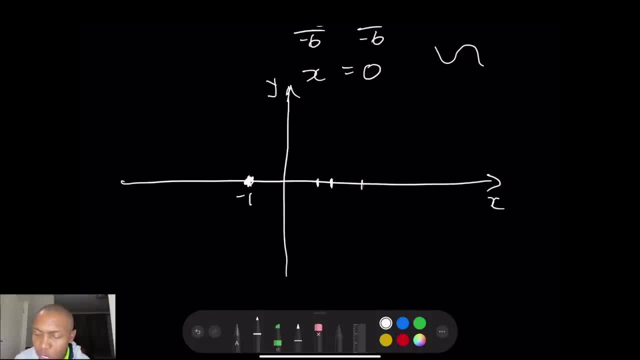 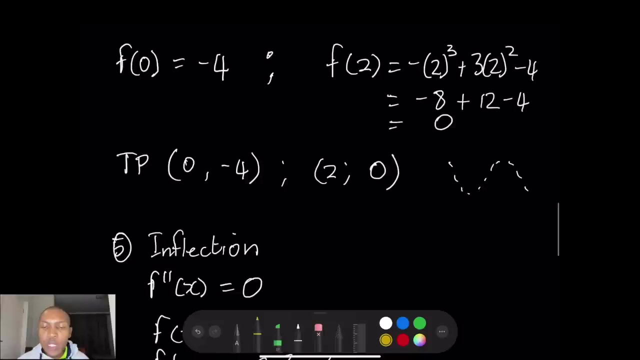 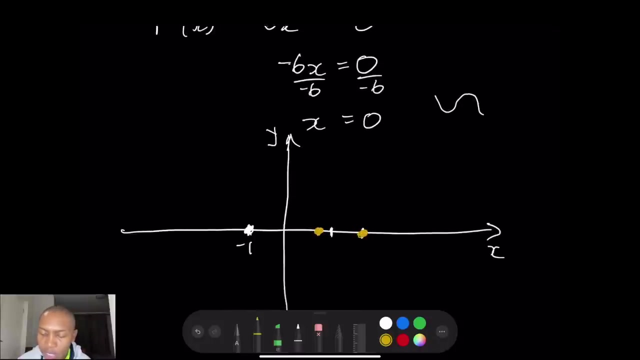 bit of space there. uh, so if we said that's one, maybe two would be over there. okay, yeah, maybe let me do that in yellow. um, yeah, let's make that one and let's make that two. okay, right now. um, now did note that. uh, in this case our turning points would be at zero and minus four. okay, so where X is, 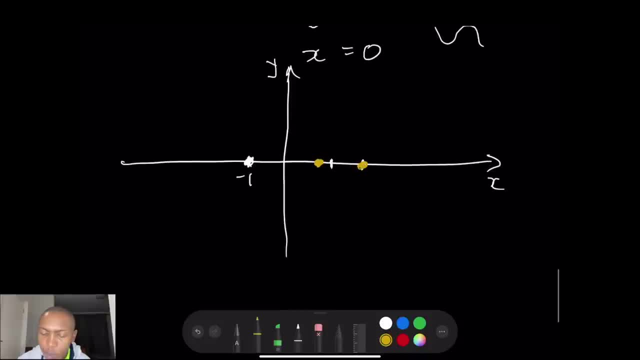 equal to zero and Y is minus four. okay, let's just say over there, okay, right. and then another one would be where X is equal to two and zero, okay. so it means I know, this is where I would have a concave up shape and this is where I would have a. 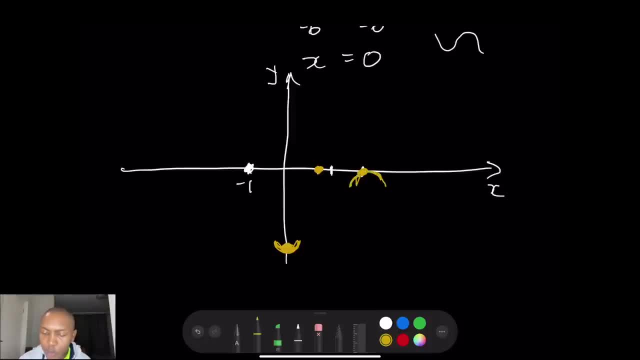 concave down shape. okay, so this is where X is zero and Y is negative. four, this is where X is two and Y is zero. okay, so, um, I think more or less my shape is coming together. all right, so now, what would the shape of my graph look like? by the way, that also, coincidentally, becomes the Y. 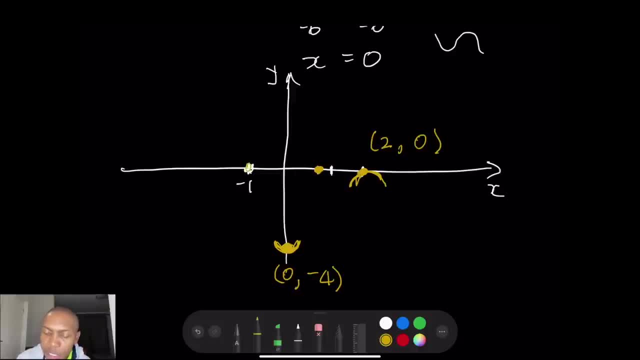 intercept as well. okay. so, what does the shape of my graph look like? okay, so, um, oh, and my inflection point. you remember this was at zero and we know that it's at zero, sorry, where X is equal to zero. so, uh, we know it's minus four as well, okay, so there, we go over there, all right, so that's the. 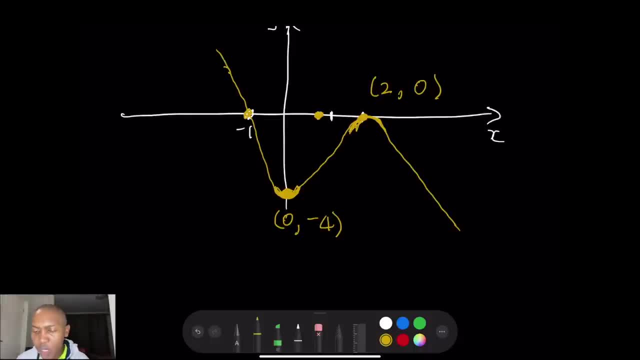 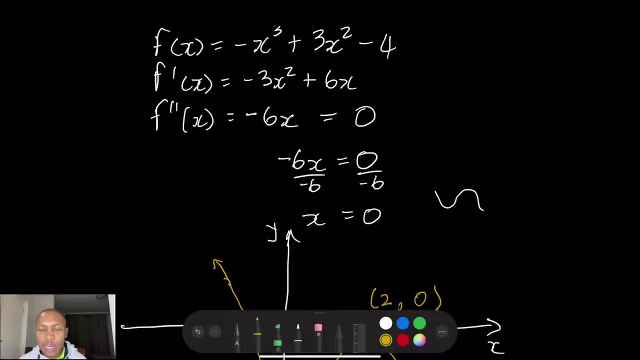 shape of our graph. that's what it looks like. okay, sorry that it looks a little bit messy, because I kept on, uh, just going over and over at the same point. so, essentially, that's what our graph would. um, this helps, ladies and gents, uh, in terms of you know, just getting a, you know just an idea of what. 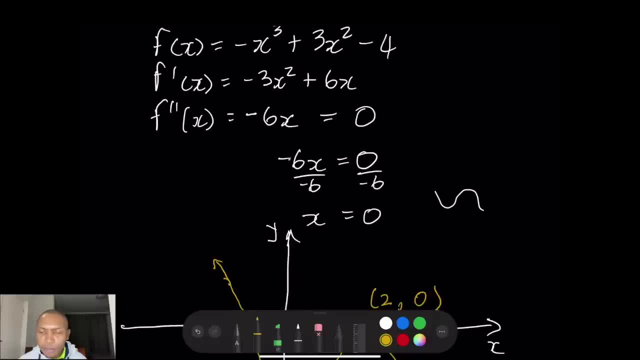 our graph would look like: um, oh yeah, actually, I realized that I had made an error when it comes to that inflection point. uh, in fact, just go back to it. uh, yeah, I see that I actually left something, all right, yeah, so, yes, it does happen in that we all make mistakes, right, you will have minus six x. uh, plus six for the inflection point. 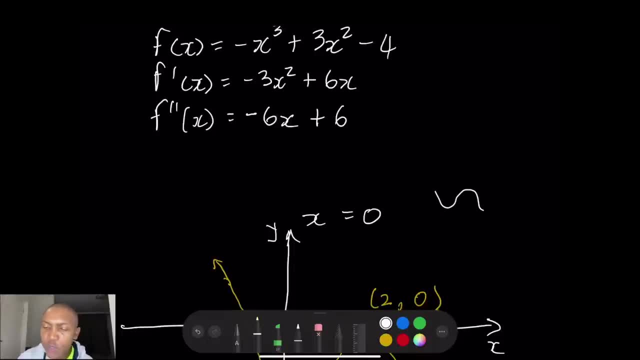 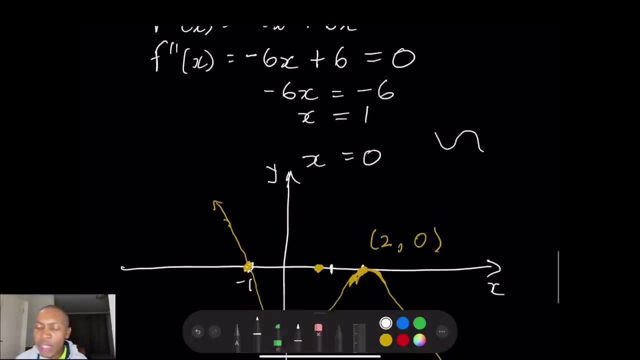 yeah, because it didn't actually make sense right? so you'd have minus Six X. plus six is equal to zero, and so you would have a minus Six X is equal to negative six, and so, of course, your inflection point will be where X is equal to one. okay, you can find out the Y value of. 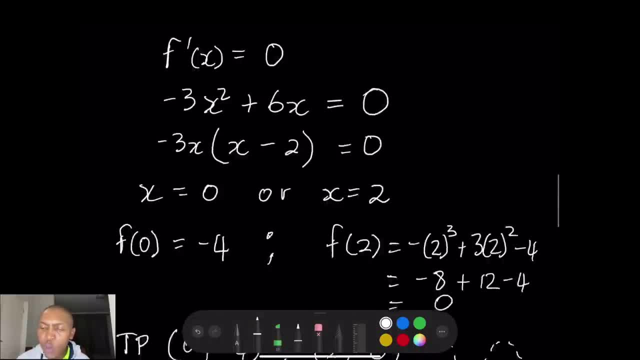 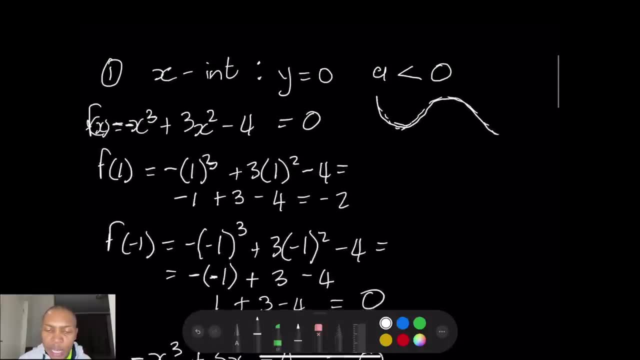 e black Vàınız Puyol, that inflection point. by substituting, I think we already have found where x is equal to 1.. You remember, when we're looking for one of those x-intercepts right Where x was equal to 1,. 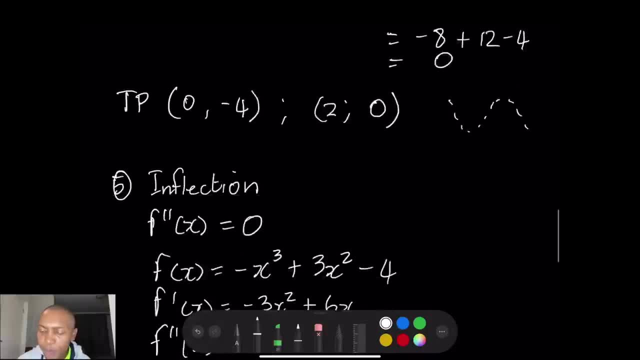 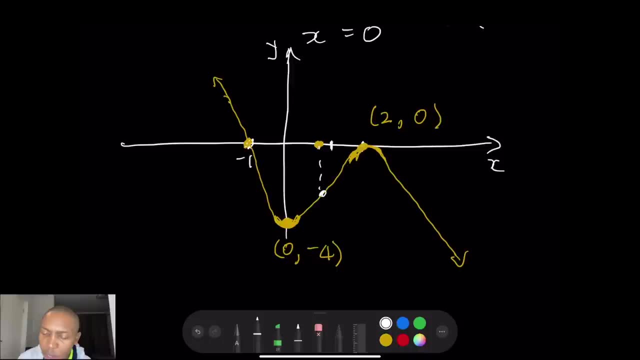 y was minus 2.. Okay, there it is. there You can substitute back. Okay, so it means we'll have an inflection point somewhere around there where x is 1 and y is minus 2.. So this would be our. 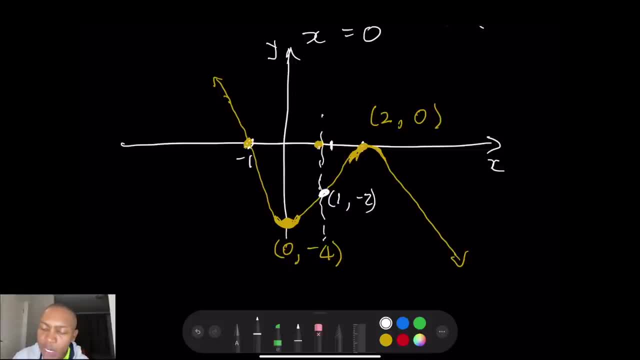 inflection point. So this means our graph: before this point here is a concave up shape, And after this point it would be a concave down shape. Okay, right, I hope that makes sense, ladies and gents, And I didn't want to actually have a long video on how to do that. So I'm going to show you how to do that. So I'm going to show you a long video on how to do that. So I'm going to show you how to do that. So I'm going to show you. 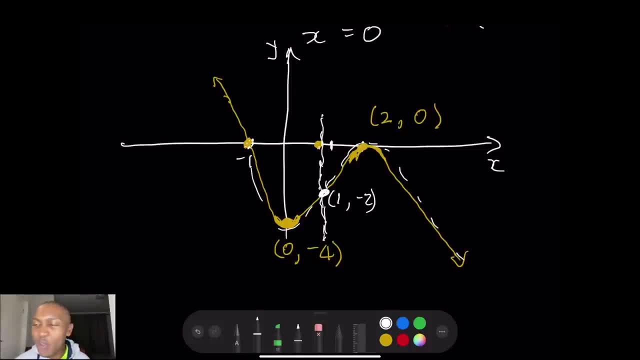 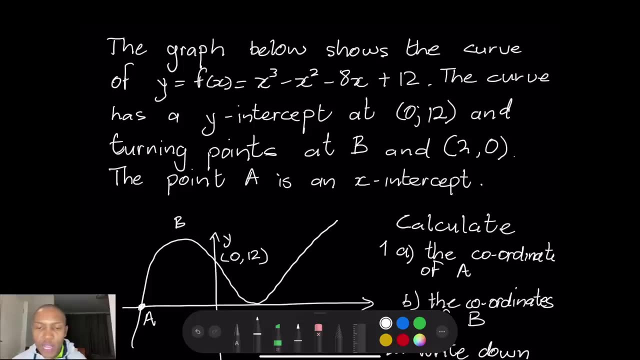 a long lesson, But nonetheless it is necessary. we have to know how to plot these functions. Let's take one last example and then we call it a day. All right, so let's look at our second example and our last one. So they say: the graph below shows the curve of f of x. is x cubed? 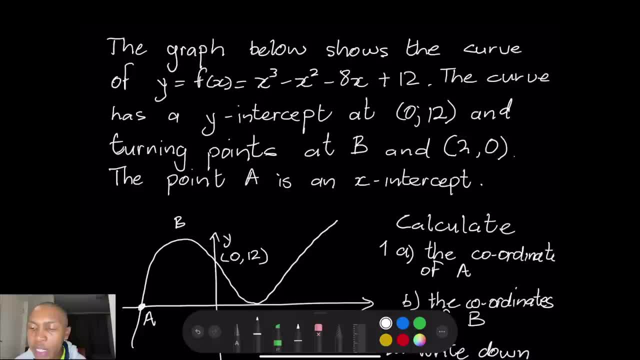 plus, or rather minus x, squared minus 8x plus 12.. They say the curve has a y-intercept at 0 and 12.. Okay, so it's that value over there. Okay. and they say they're turning points at b. 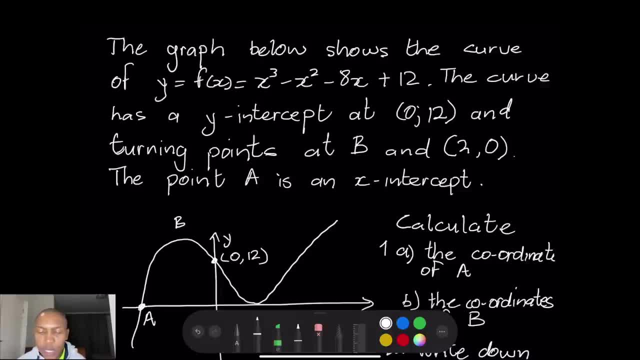 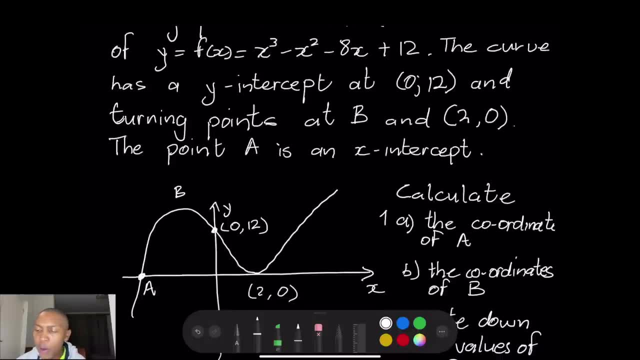 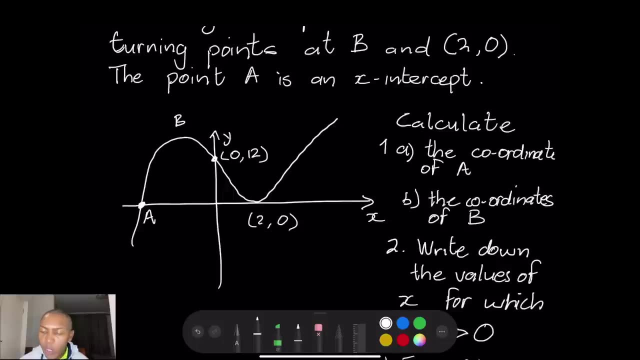 and 2 and 0.. And then they say: the point a is an x-intercept, So point a is over there, All right now. they say: calculate the coordinates of a Right now, to get the coordinates of a, what we would need is a coordinate of a. So we would need a coordinate of a. So we would need a. 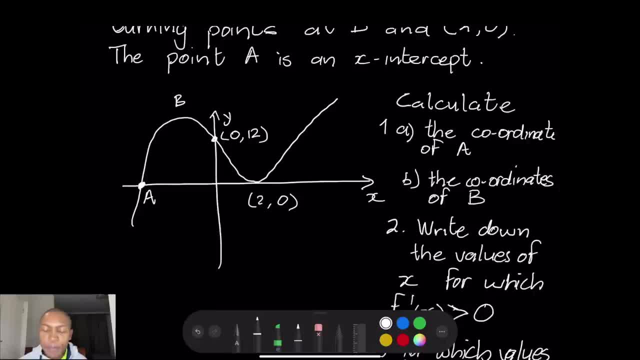 coordinate of a. So what we need to do is just try to find, obviously, the x-intercept. But I want you to please note, ladies and gents. they said this point here is a turning point. But can you see that it's a turning point, but it is also an intercept, Okay, so it is actually turning. 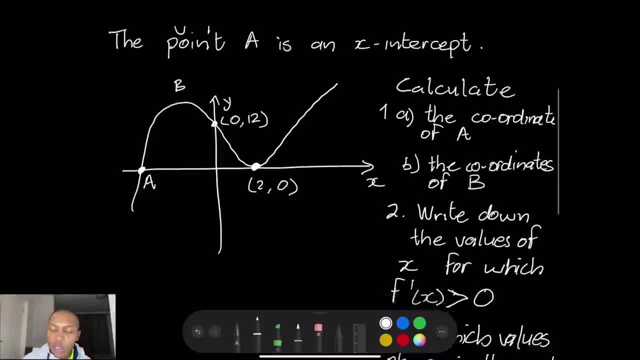 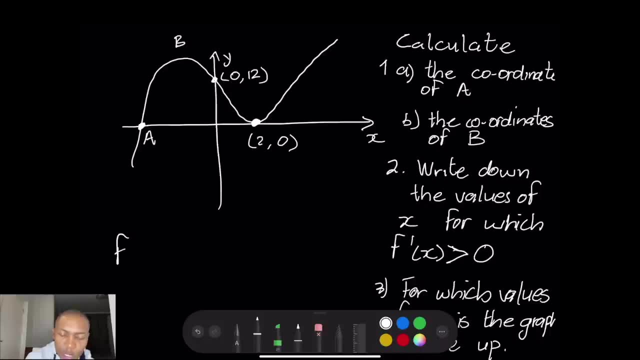 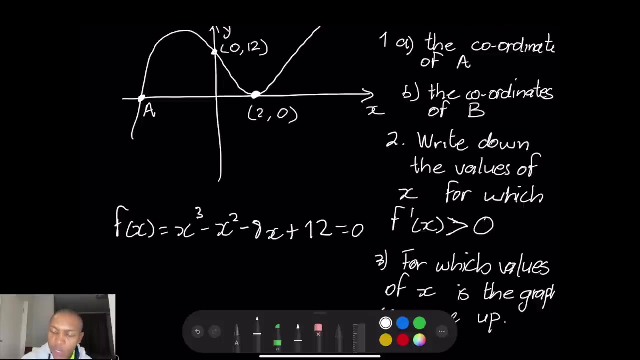 there, but it's also an intercept, So what it does is that it actually enables us. okay. so I'm just going to say: well, f of x. we said this is x cubed minus x squared minus 8x plus 12.. Okay, right, So that means okay, which is equal to 0.. Okay, so that we don't. 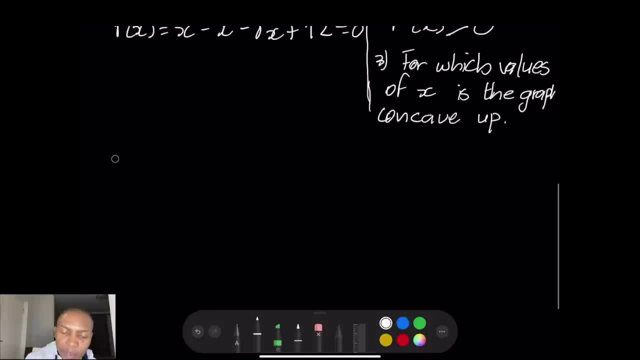 actually, yeah, maybe let's just write it down. Okay, so we've got f of x, which is equal to x cubed minus x. squared minus 8x plus 12 is equal to 0.. So let's just quickly do that there. So remember once the values where. 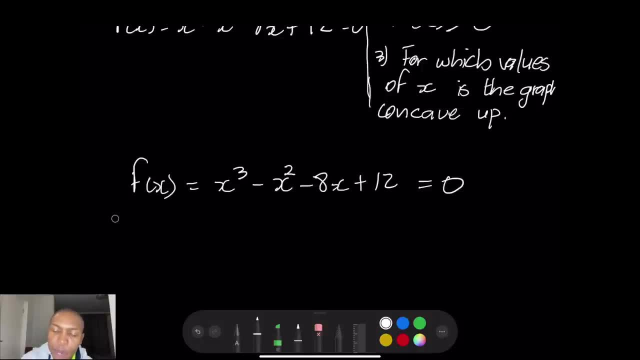 x is equal to, or rather f of x is equal to 0, but we already know that x, that turning point at 2, there is one of the factors. So I'm just going to say, well, x minus 2.. So let's get the. 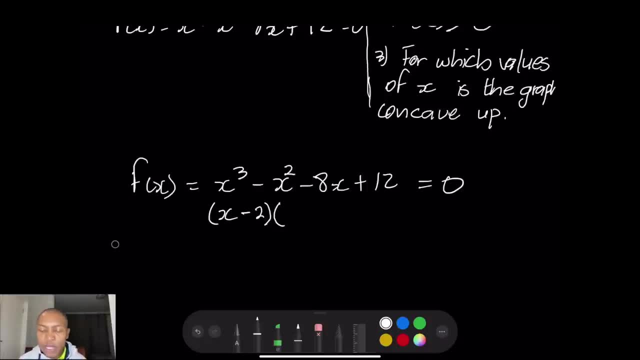 other, you know point in this case. So we know this would be right: x multiplied by what will give me x cubed, So that will be x squared. And I know for the last one, minus 2 multiplied by what? 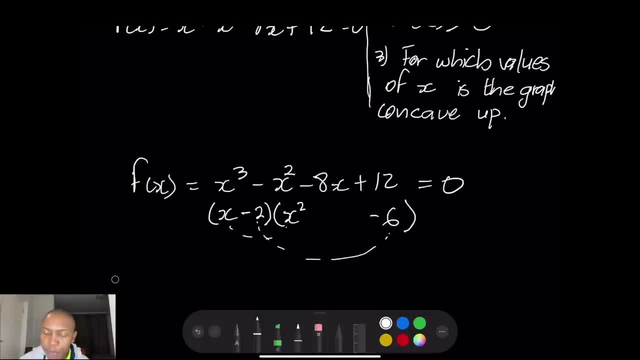 will give me x squared. Okay, so to get the middle term. so I know I already have minus 2x squared. minus 2x squared, All right, But my final result is minus x squared. So what do I need? 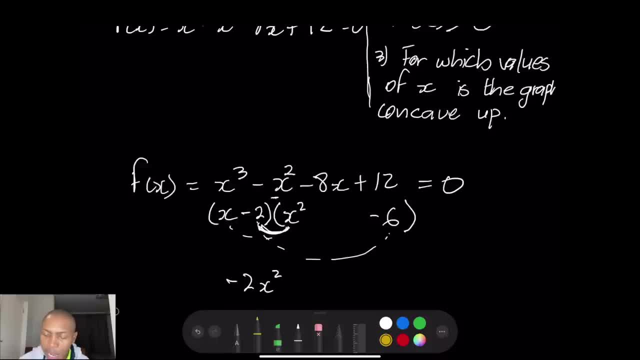 I need in yellow. I need a plus x squared so that minus 2x squared plus x squared will give me that minus x squared there, right? So I need to create this minus x squared. So question is: x in the yellow multiplied by what will give me x squared? And the answer is: 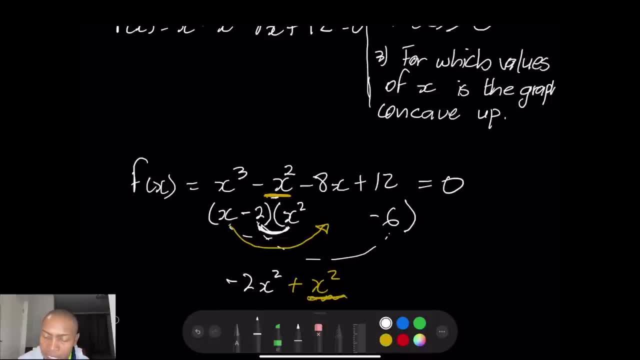 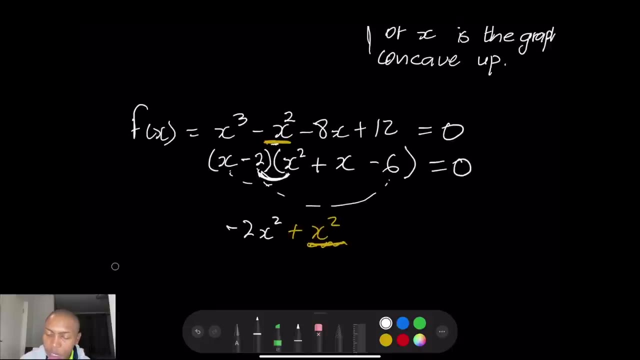 quite simple. That will be plus x. Okay, so that will be plus x. So this will be plus x, And this will be equal to zero. Now let's factorize the rest of our quadratic function or equation. rather Right, so you've got x minus 2.. 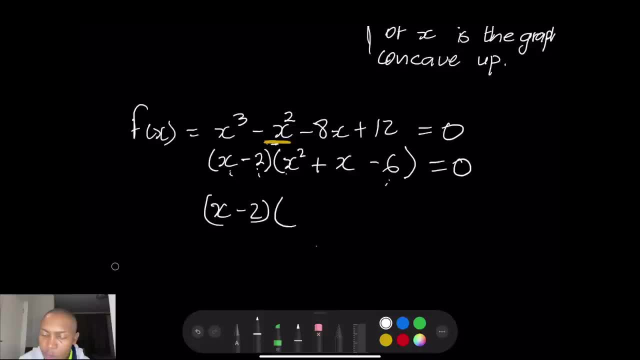 Right, if I factorize this here, this will be x plus 3 and x minus 2.. Okay, right, So you can see those are the same there, And that's that turning point, as well as the x intercept. So it means that the point A would be: x is equal to minus 3,. 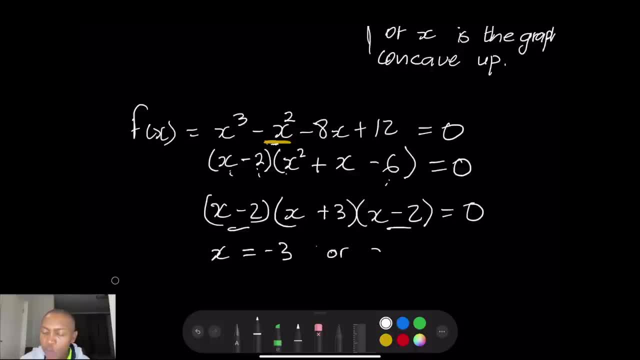 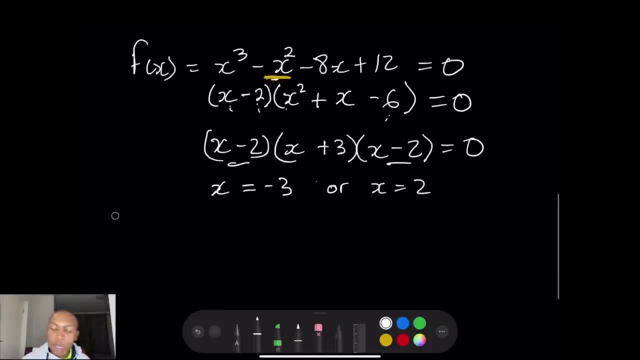 right. And the other one, remember: x is equal to 2.. We already have that. They had already given that to us. Okay, so in this case, it means that A would be minus 3.. And the other one, remember: x is equal to 2.. We already have that. 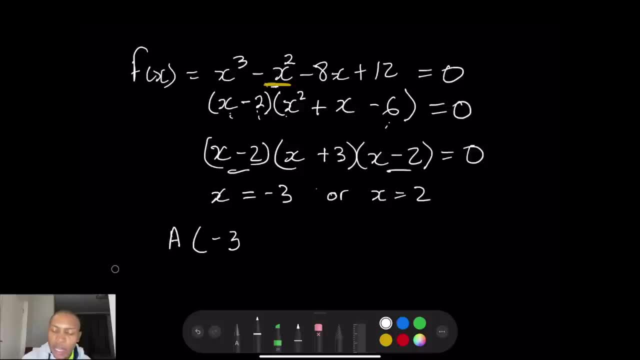 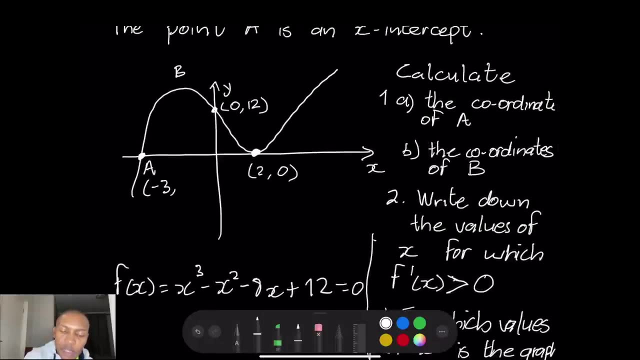 It would be minus 3 and 0.. Okay, so if we go to that graph there, it means that's minus 3 and 0. Those are the coordinates of that point A there, Right? and then they are looking for the coordinates of B. And remember what did they say about B? They said B is actually. 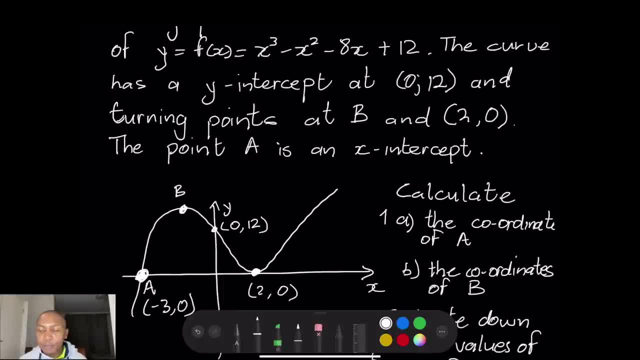 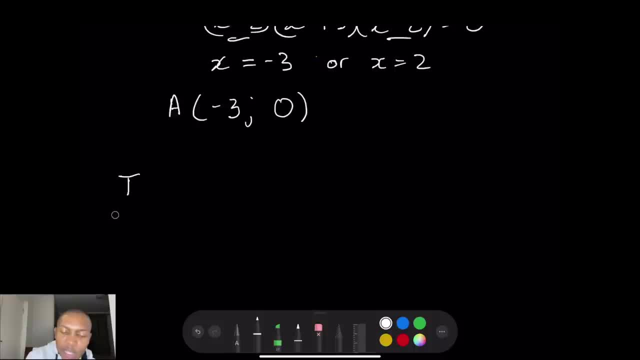 one of the turning points. All right, Yeah, they said the turning point is one of the turning points. The turning point is at B. So how do we get the turning point? Remember, we said, to get the turning point, you simply take the derivative and make it equal to 0.. Okay, so now remember our f of. 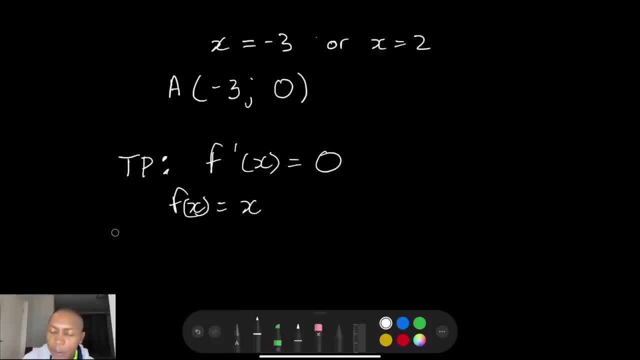 x was x cubed minus x squared. Okay, minus 8x plus 12.. So this simply means f prime x. Okay, we're taking the derivative. This is going to be 3x squared minus 2x minus 8.. And this is equal to 0.. 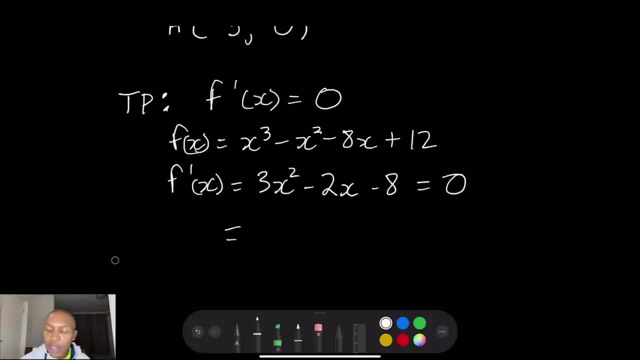 Right Now, of course, this is where you're going to factorize. Okay, so we are looking for factors of 3.. That's easy. That's 3 and 1.. Okay, we're looking for factors of 8.. Okay, such that when 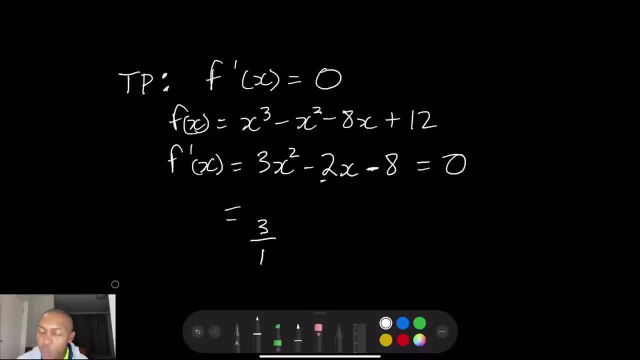 we subtract them, they give us negative 2.. So, factors of 8, let's try 4 and 2.. Okay, let's see if I cross. multiply that 3 times 2 is 6.. 1 times 4 is 4.. And of course, 6 minus 4 will give me 2.. 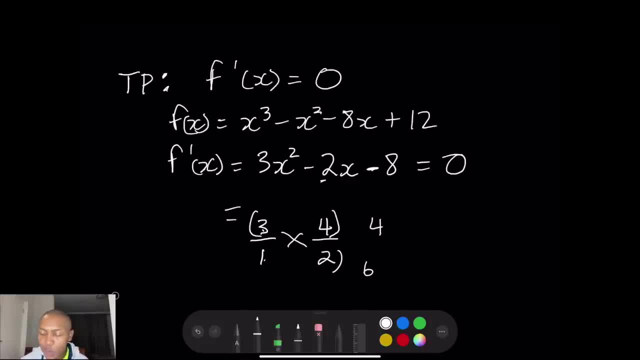 So it means this is my first bracket And this will be my second bracket. Okay, Right, Oh gosh, Okay, so this will be. we said okay, so that will be x and 2.. And that will be 3x and. 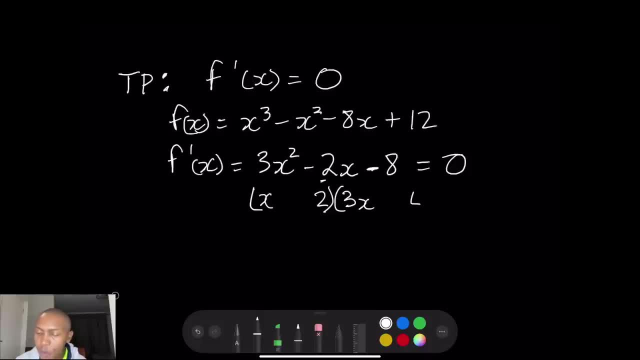 4.. Okay is equal to 0.. Okay, so in this case we're going to take the derivative of x squared. Remember my, you know, the bigger product must take the sign of the middle term. So my bigger. 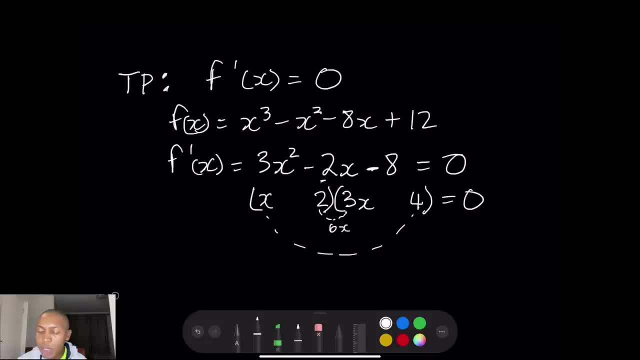 product in this case would be 6x. 2 times 3x is 6x And in this case I've got 4x with that one. So which means that 6x has to be negative. So that's negative And that's positive over there. 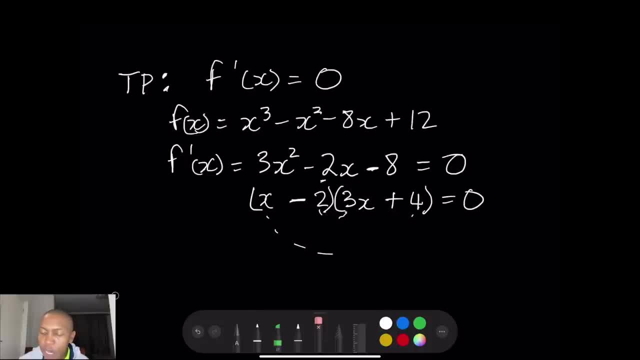 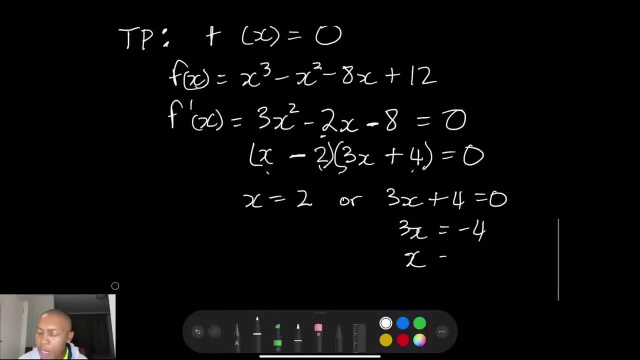 All right Now. so which means this is at x is equal to 2.. Or this would be: 3x plus 4 is equal to 0. And 3x is equal to negative 4. And therefore, x would be minus 4 over 3.. Now, of course, to get the y value. 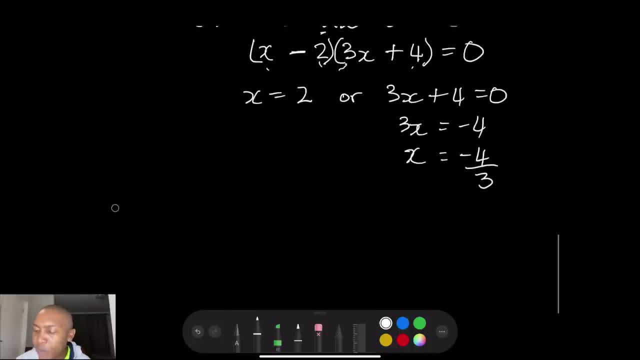 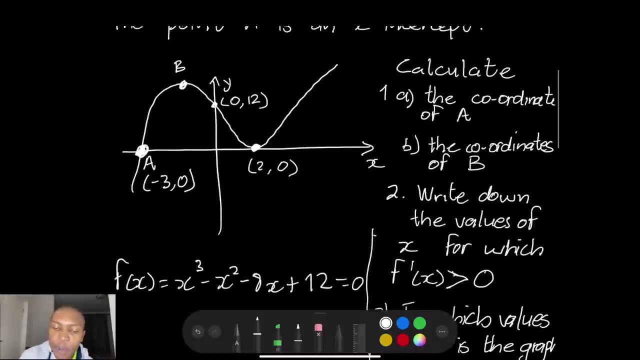 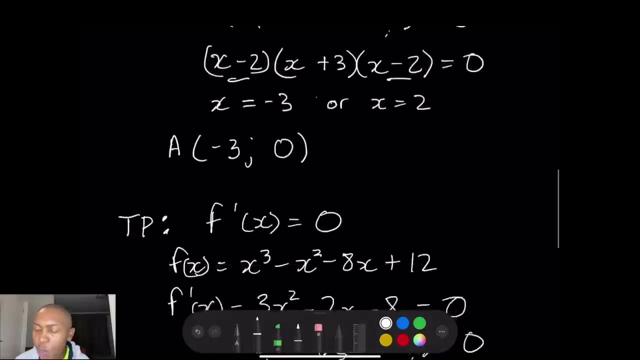 of our turning point. we're going to take that x value So, which means that's the other turning point. we already have that one which is at 2 and 0. But we want the one at b. we already know that the x value is that value that you got minus 4 over 3.. 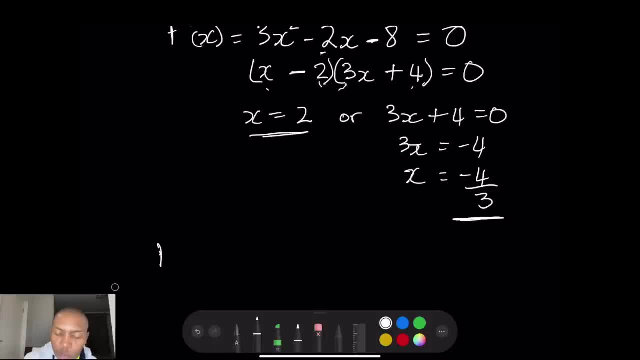 Right. so we're going to take that and say: to get the y value, that's minus 4 over 3, f of minus 4 over 3.. So this is going to be minus 4 over 3, cubed minus a negative 4 over 3, squared minus 8 times minus 4 over 3 plus 12.. 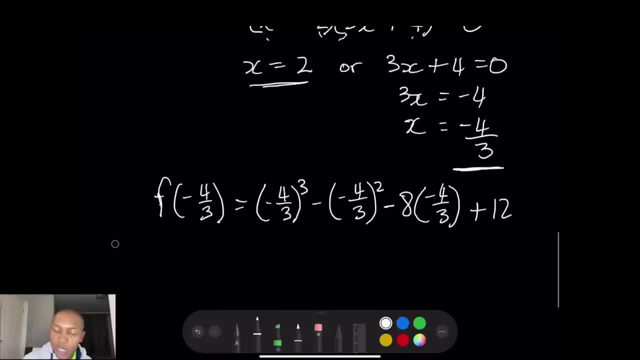 Okay, I'm just going to put that into my calculator quickly. Okay, so I have got 4 over 3,, 4 over 3, okay, so negative 4 over 3, so that's cubed. okay, Ooh, I'm making so many errors here. Cubed, that's minus. again, that's negative. 4 over 3,. 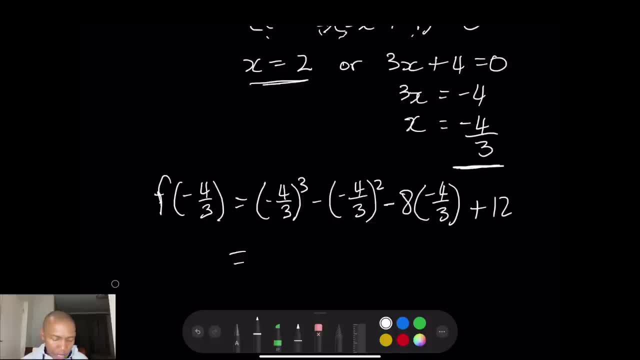 that's squared, that's minus 8 into 4, over 3, okay, Oh no, I almost forgot that. negative again plus 12.. Okay, you can verify that with me. ladies and gents, I get a very strange value. 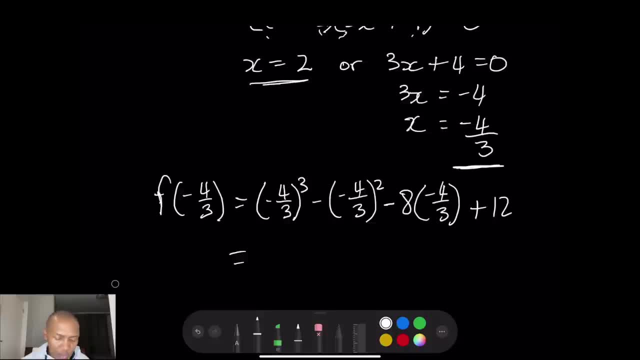 Okay, 18.52, or you can round it off as 500 over 27.. Okay, if it is incorrect, please you can correct me. comments: uh, five, two, so in this case i've got minus four over three, uh, which is 18.52, or if 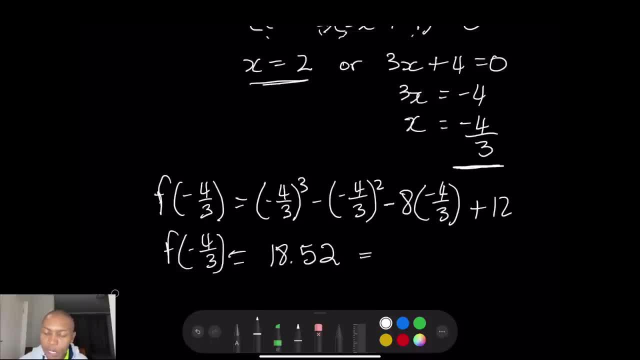 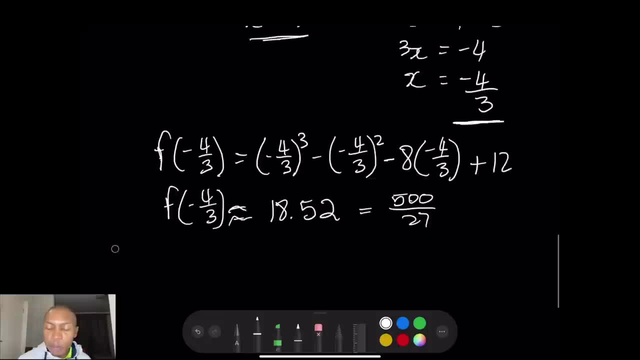 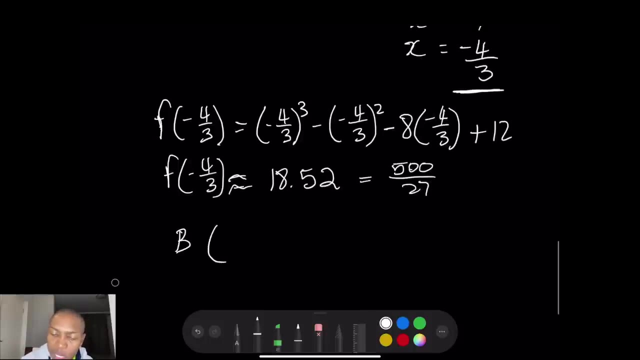 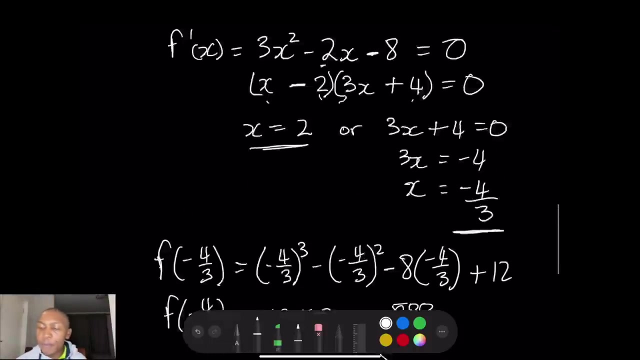 you want to. um, so this is approximated to that, or accurately, it's 500 over 27. okay, right, so it means that the value of b- all right- would be actually that minus four over three, as well as 18.52, and it makes sense. it's a positive y value and a negative x value. all right, now let's go right. 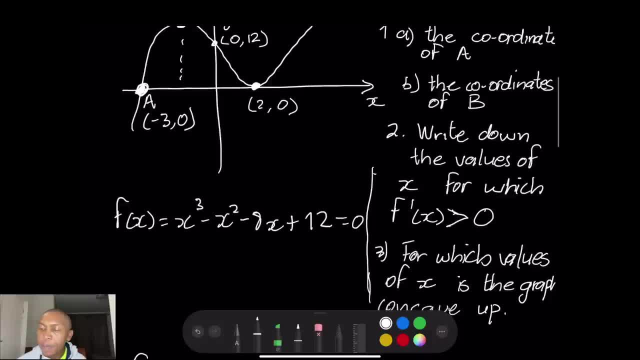 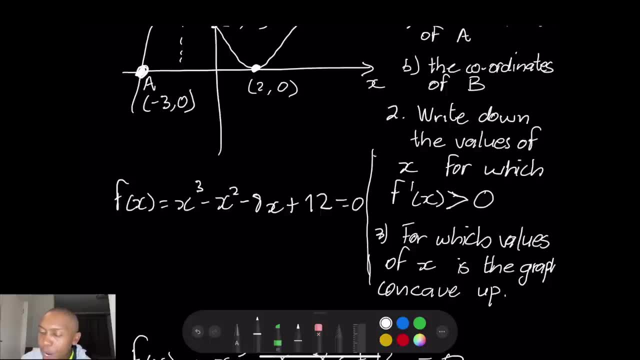 into it again. um, so the second part. they said: write down the values, for which- the values of x rather, for which- f prime x- the gradient is greater than zero. and we must be very careful here, right? um, in this case, what it simply means is we're going to look at our graph and say: 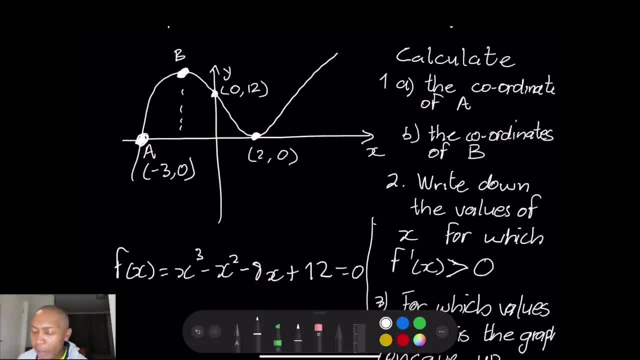 well, where is our gradient greater than zero? okay, so where is our gradient positive? i want you to please note so: everywhere, from infinity, my gradient is positive. until b. b is has a gradient of zero, then it starts becoming negative. right, and then you can see that it's zero here, but then it starts. 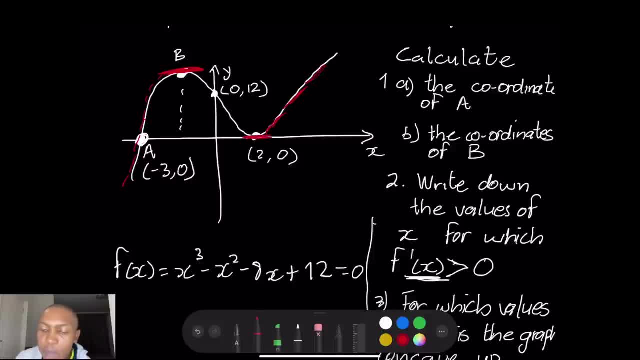 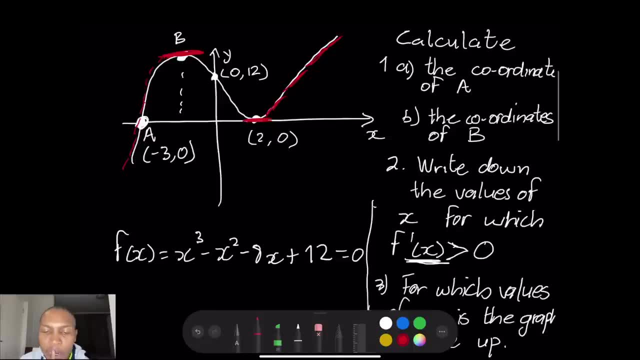 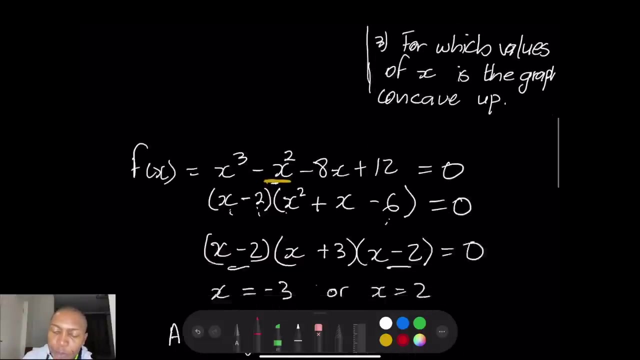 becoming positive again. okay, the steepness of the graph starts becoming positive after two, right. so what are the x values where the gradient is positive? from negative infinity right up until that turning point which is minus four over three, and then it's from two to infinity- right. so we can say: well, in this case, this is how we're going. 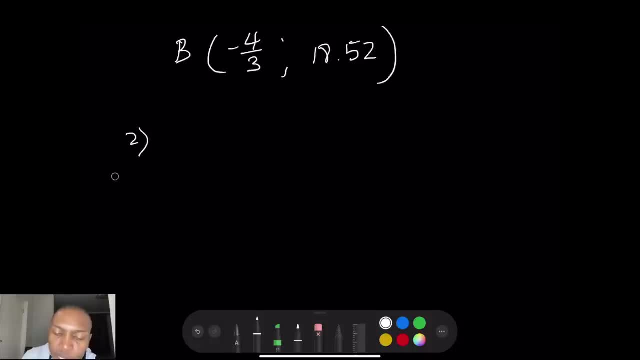 to write it out. okay, we can say: x is an element of minus infinity. we never include that up until minus four over three. but do we include it? no, and the reason for that is that, remember, at minus four over three it's not positive, it's not greater than zero. if they said greater or equal to, then we would include that. 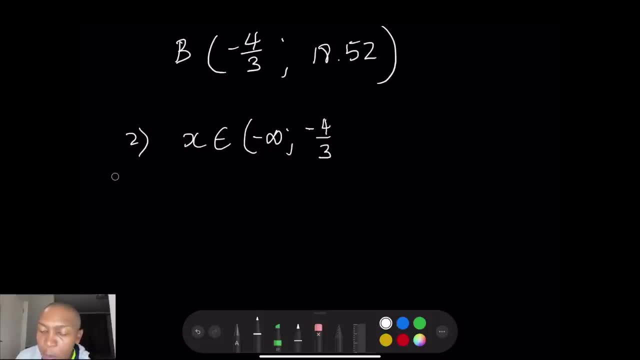 value, but at minus four over three it's zero, but we want only greater than so we're going to exclude that value, okay, and in this case in union with okay. so again we said: from two, okay, we exclude two, because at two, remember, it's zero and till infinity. right, so till infinity. of course, you can write that as: 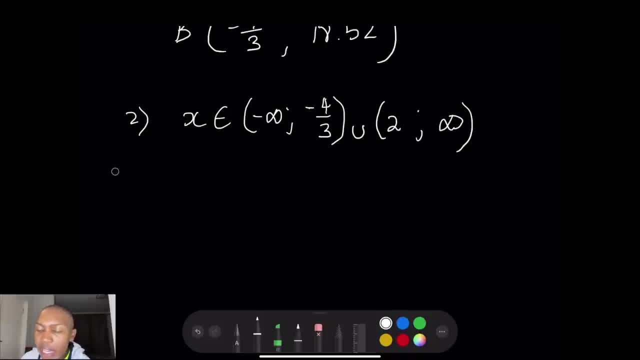 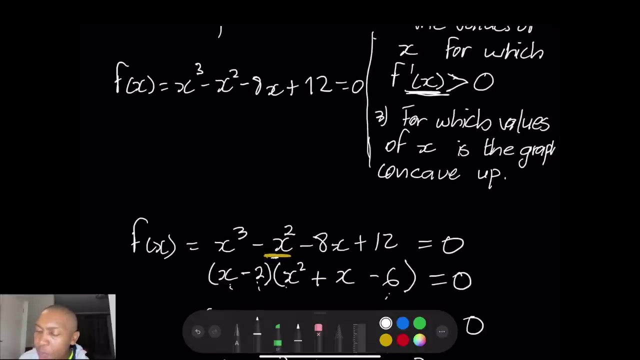 for values where x is less than minus four over three and for x greater than two. okay. for any values greater than two, all right, okay, uh, the last portion. they say for which values of x is. the graph concave up right now. in this case, again, how do we work out? 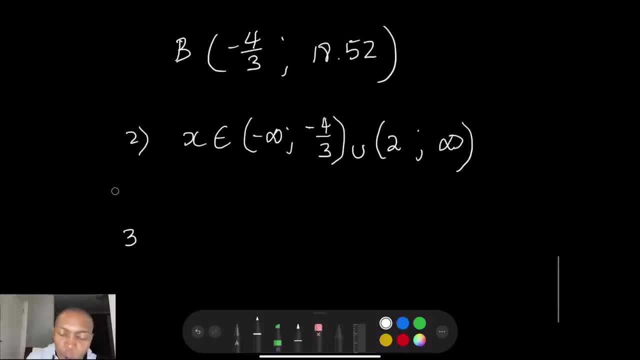 whether a value is concave up, or rather, where the graph is concave up, it means that we need to find the point of inflection right. so we said okay. so f of x. remember, this is x cubed, okay, minus x squared, minus 8x plus 12, all right. so we said okay. so f of x. 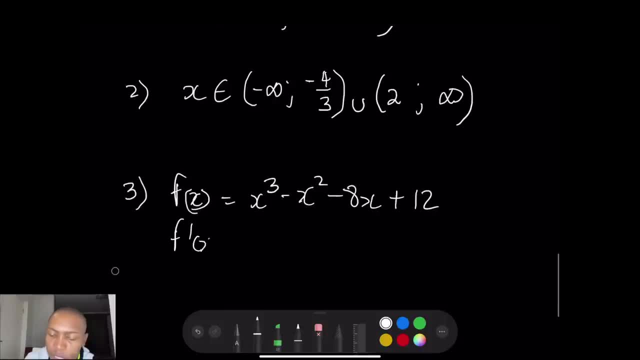 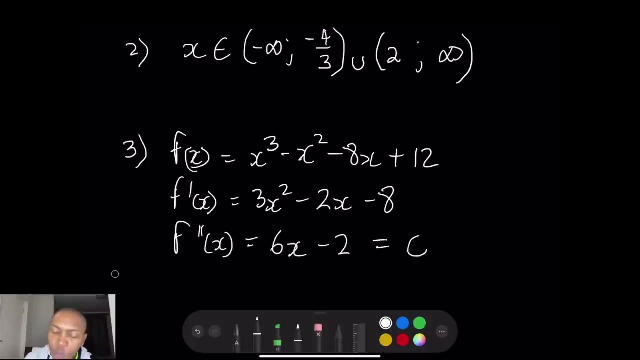 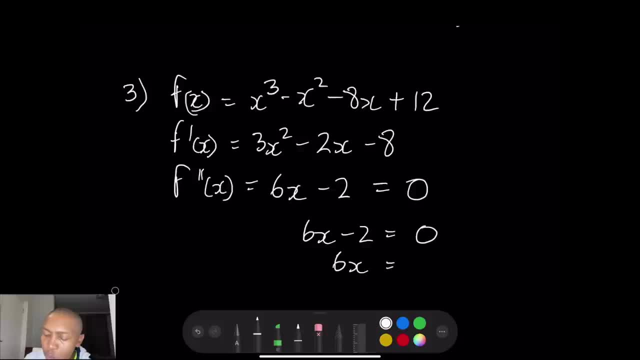 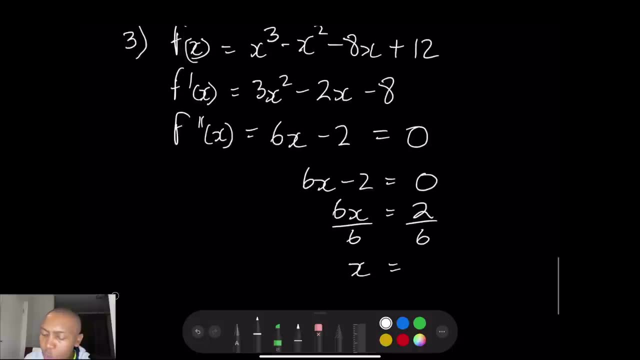 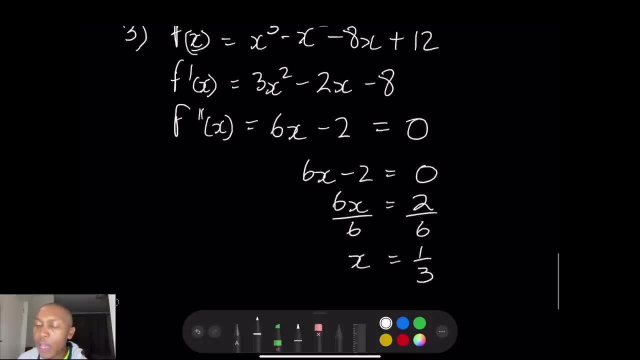 and so 6x is equal to 2, and if we divide that by 6- okay, so we know this would be at- x is equal to 1 over 3. now they were looking for the x values where the graph is concave up right. remember that. 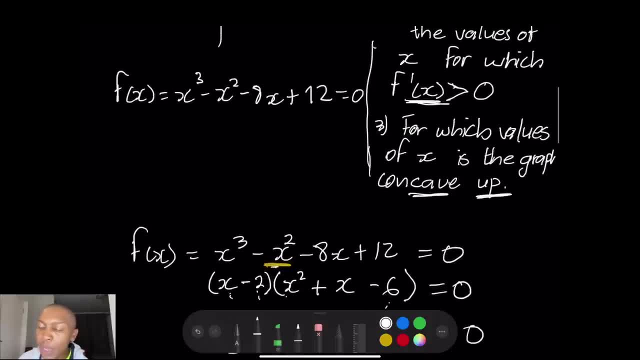 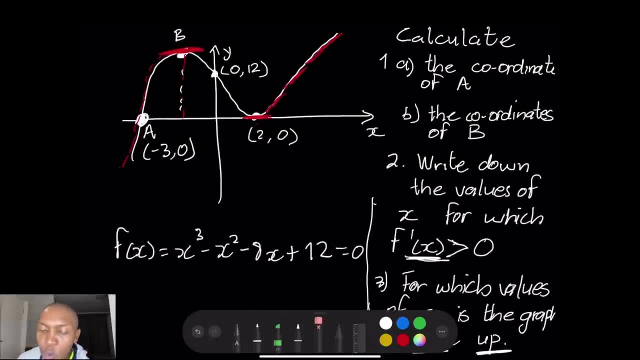 that was our question, concave up, remember, at the point of inflection. we know you can see there. so it means from 1 over 3. okay, so i mistakenly just deleted that there. okay, so from 1 over 3. okay, so that was our graph, right there. okay, so, from 1 over 3. so we know, in this case, that would. 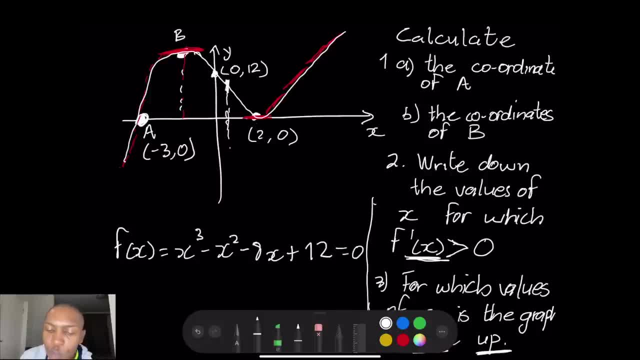 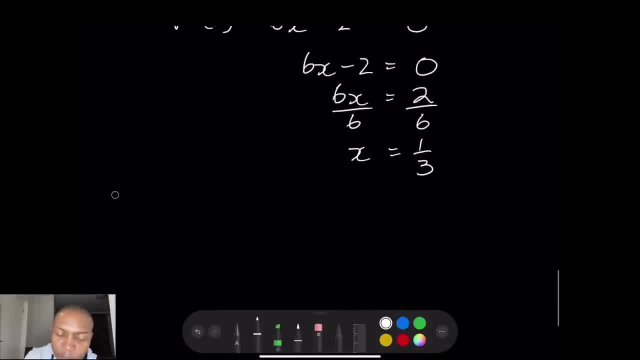 be a point of inflection, so it's concave up from 1 over 3 right up until infinity. so we can say to answer that: okay, safely, this is x is an element of 1 over 3. okay, in this case. so that's from 1 over 3 up until infinity. okay, right, again, we don't include that. 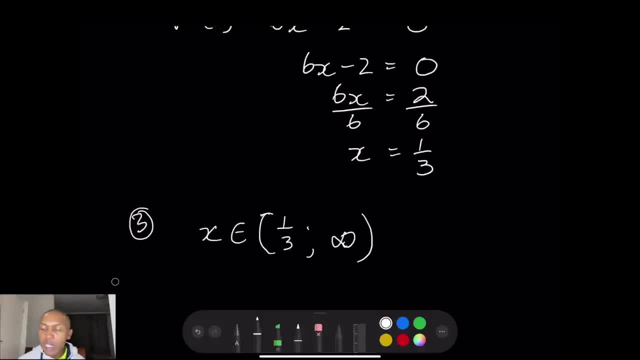 value at 1 over 3 there, all right, and essentially that is how the cookie crumbles. now, ladies and gents, i know this is a very difficult question, but i'm going to give you a little bit of a little bit of a lengthy lesson, but of course, it is worth it when it comes to cubic functions.